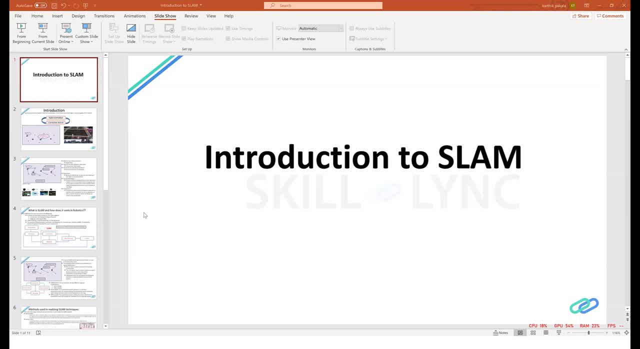 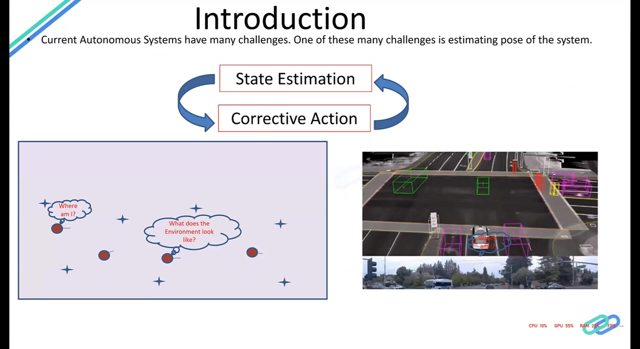 vehicles or autonomous robots or any such autonomous applications are very vital and, you know, pretty fast rate in today's world. One of those systems that we are talking about today is SLAM, which is nothing but simultaneous localization and mapping, which is one of the primary components of these autonomous systems. So let's go ahead and start with it Simultaneous. 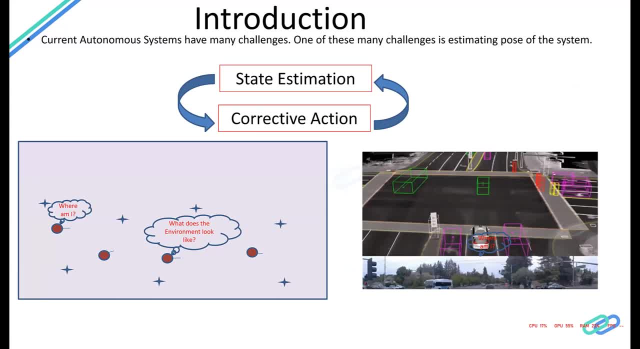 localization and mapping, For example. let us think about ourselves. What do we need to know and let to know. what do we need for us to understand where we are at and how we see ourselves to be at any given location? We need to know the surrounding, and we also need 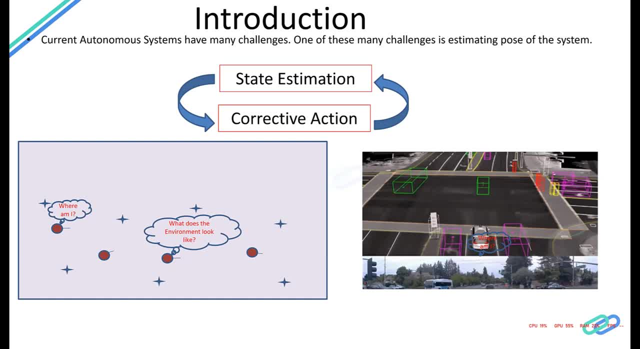 to know where exactly we are in that surrounding. That is exactly what is being done for a robot using the SLAM systems. If you look at the state estimation and the corrective action, what does those mean? State estimation is the state estimation of the robot. The state estimation of the robot is: 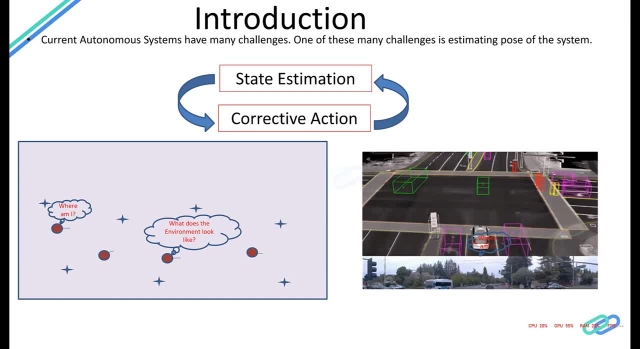 defining what what state you are in, or it will define where exactly you are supposed to be in and you know where are you at currently. So that is defined by the state of the system, and corrective action is nothing but the action that is taken based on the algorithm that you have, the SLAM. 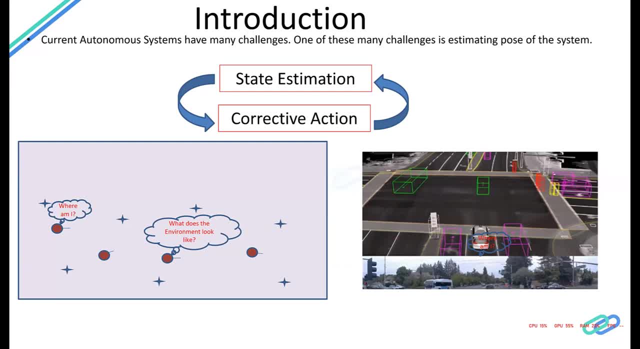 algorithm that you have to correct the system's action and put it in the right pose, as you intend it to be. This is where, like so here is where the algorithm comes into play. right, The corrective action and also making the robot aware of its current position is where the SLAM 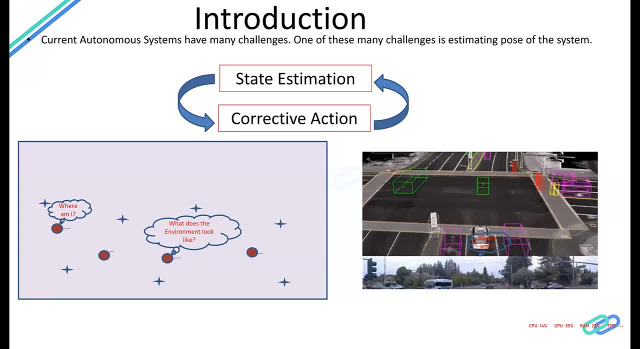 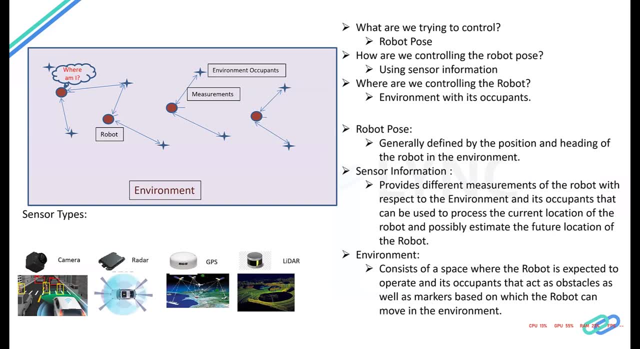 algorithms come in. So let us go into the next part of it. So here is an example that I'm taking, where you have a robot in a given environment and you have different components of the environment. Let's say they're environment occupants. So what are environment occupants? For example, let us take 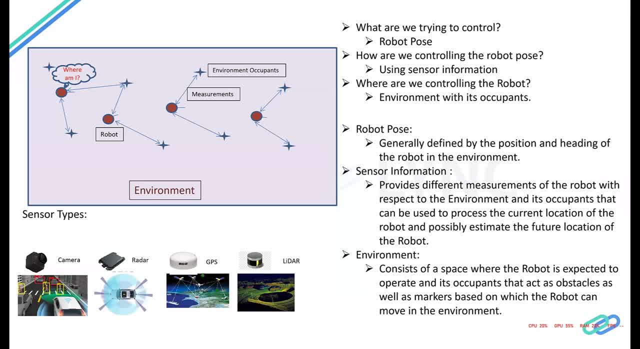 an example of autonomous way. You have an autonomous vehicle. You have different other cars on the road as well along with you. that is one of the environment where the component occupant and you have the traffic lights that a car is trying to read. That is an. 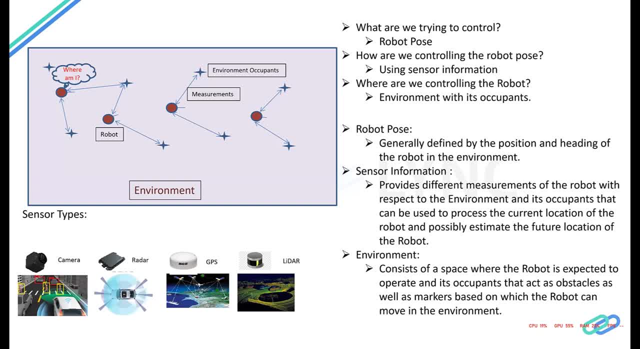 environment occupant. So all of these different components that are comprised within the environment are termed as environment occupants. So how does the robot perceive itself when it is in a given environment? it needs some kind of an information, right? so before we go there, let us talk about the robot pose. what is the robot pose? how do 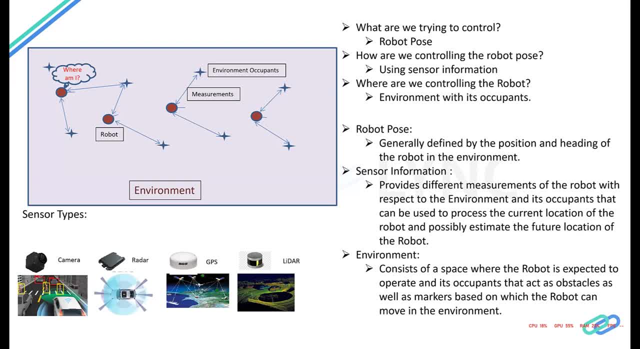 we define it. a robot pose is nothing but it. it it is the characteristic of the robot that will give you the position and the heading of the robot, which means that for any robot, if you take any example, whether it's a humanoid robot, whether it's autonomous vehicle, whether it's an undersea robot, whatever it might, 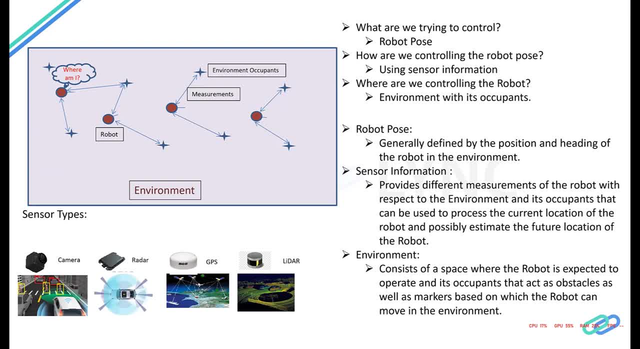 be two of the major components that you can always rely upon. to you know, tell the system that it is at a given location, is your heading, and distance, and distance with respect to the environment occupants, the other environment occupants. I'll go into detail in that regard in the next slide. 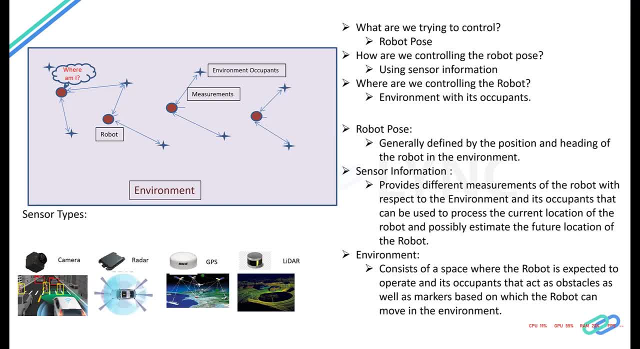 also- but this is the brief introduction of what the robot poses- now, coming to reading the environment. how can you read an environment? you need to have some kind of a way to perceive the environment, right? so that's where the sensor is coming to play. so you have different types of sensors that you have access to. 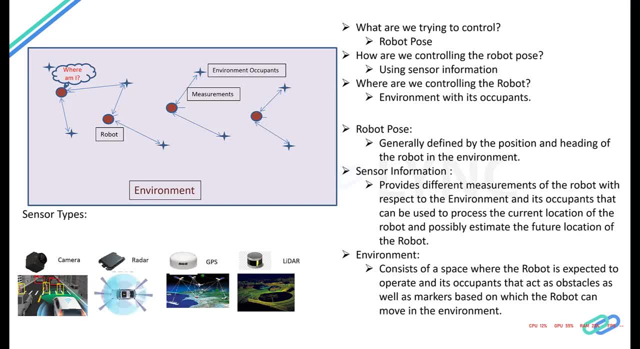 today that can read the environment in different ways. for example, if your examples have been given below, which are camera, radar, GPS and LiDAR, each of these different sensors give you a certain perception of the environment, which will help you localize and also map the environment that is around you. each of these can be used for a different function and also. 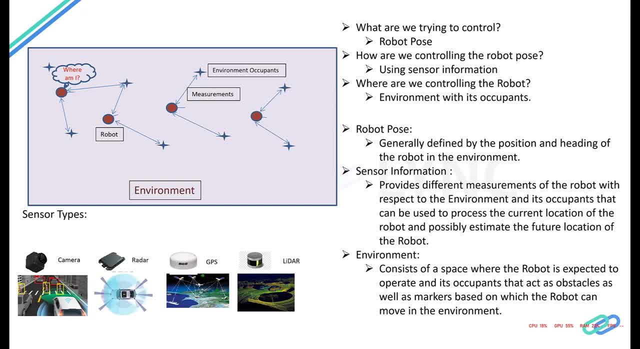 you also have something called sensor fusion, which will help you to use the signals, use the data that is coming in from all these different sensors. you know, in a collective way to perceive the environment and you know, localize yourself or the, localize the robot in the environment. let's move on to the 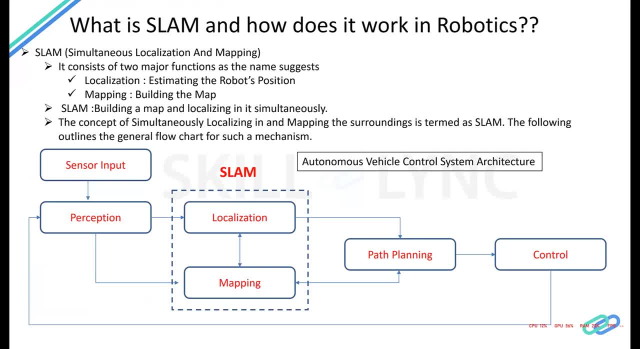 next one. now you understand, with the introduction of what you're trying to do here with respect to the SLAM algorithm. let us understand what is SLAM first right. so, for what we've talked about is: what are the system that we are dealing with? we're dealing with robotic systems that need to be localized and also map. 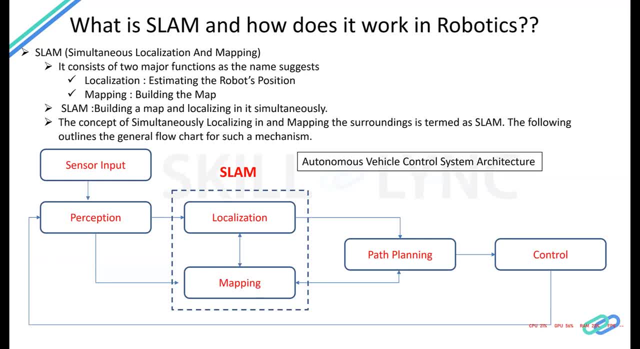 the environment. so you can say: or you can basically create a way for the robot. you can say: or you can basically create a way for the robot, you can basically create a way for the robot. you can basically create a way for the robot to you know, let it. let it know where it is. 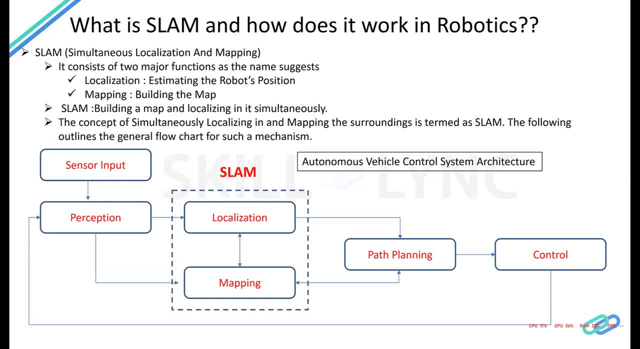 located it in the given environment. That is the basic functionality of any given system, whether it's a living being or whether it's autonomous vehicle. whatever may be the system, this is one of the major functionality that we always look to. So let's talk about FLAM systems. FLAM is nothing but simultaneous localization. 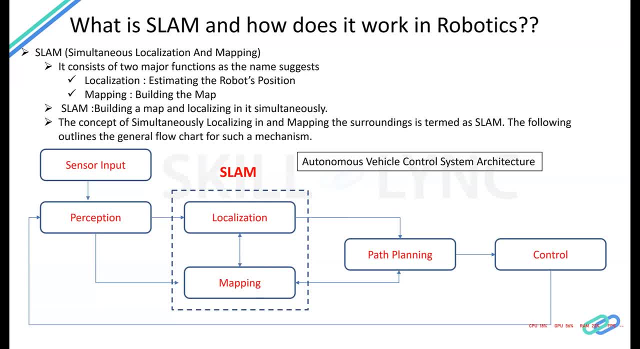 mapping, as I've talked about already. So there is, as the name suggests, there is, two major components in a FLAM system: One, localization and two is the mapping. What is localization? So let's talk about localization. Localization is nothing but put yourself on the given map, Say where exactly you are at. So localization is a. 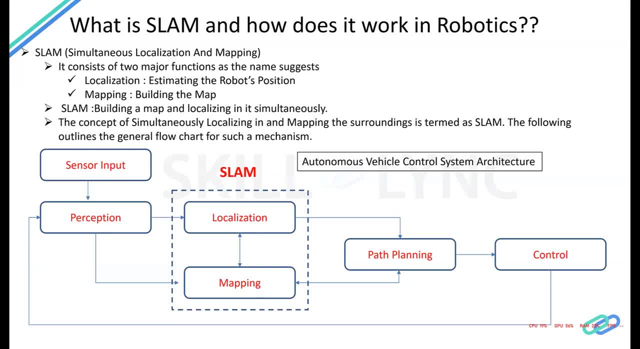 function that will tell the robot exactly where it is located: it on a given map. When I say map on a given environment, So environment is defined by the map, right? So, for example, let's talk about Google Maps. I think you already, you do use it. 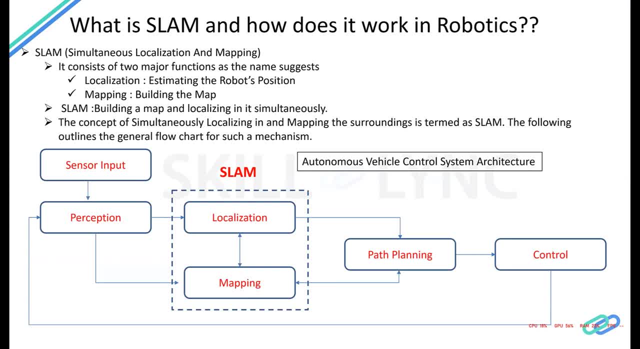 on a very regular basis. So what this Google Maps do? It will put you on a certain location based on different sensor input Right, One of which is a GPS sensor, Like we talked about earlier. You are perceiving the system or you are. 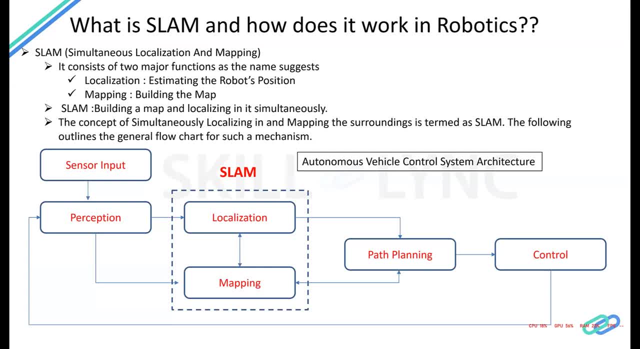 perceiving the input or you are perceiving the environment to the robot to tell you exactly where you are based on certain sensor information. the sensor information in case of google maps is coming from a gps sensor: right localization gps information helps you put your, helps, put yourself on the map so that the robot can perceive as to where exactly it is. 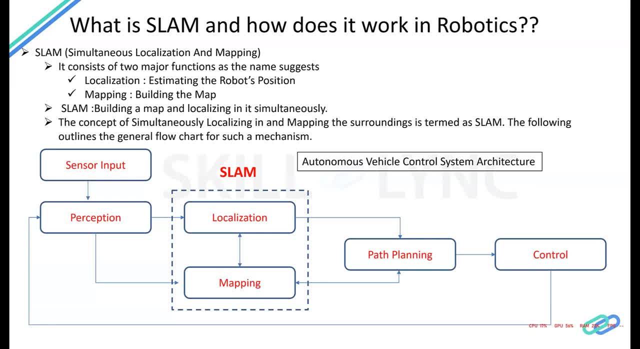 located on the given map. right, google maps is like a really huge map. it's pretty big, right. but how about a system? let's take an example of an indoor system like your home, right? in that case, you don't really have google maps right, so you need to be able to first look map the system or the map the. 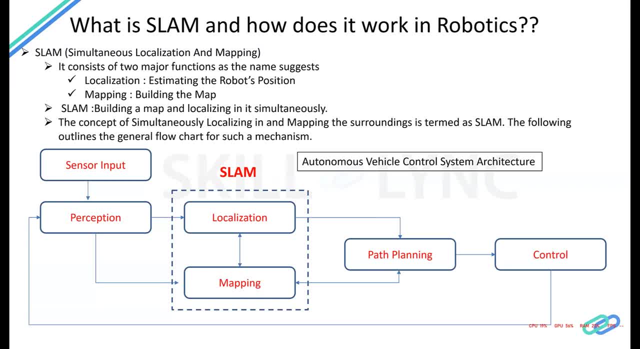 environment. number two localized object or the robot that you're trying to localize in that environment. here is the example, or here is the generic system architecture as to how the system is designed when it comes to slam systems. okay, so first, for any robot, it has to have some kind of a way to perceive the environment. 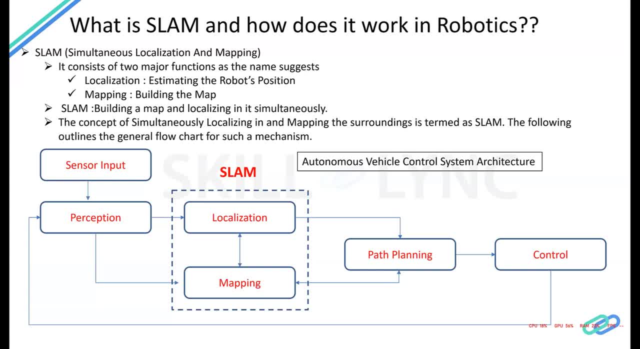 so that is what is the sensor input represents. so it can be any type of sensor, right? uh, a few examples that i've given earlier we'll talk um. we'll give you a brief idea of what types of sensors that we use on a regular basis, but let's not go into details of the sensor types. 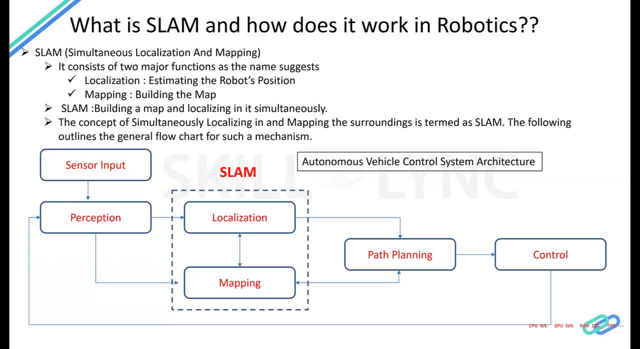 but let's just stick to the system architecture that we're talking about here. so you have a sensor input. it can. it can be a gps sensor, it can be a vision sensor. it can be in a state, can be. it depends upon the function that you're trying to write and what kind of environment you're in now. 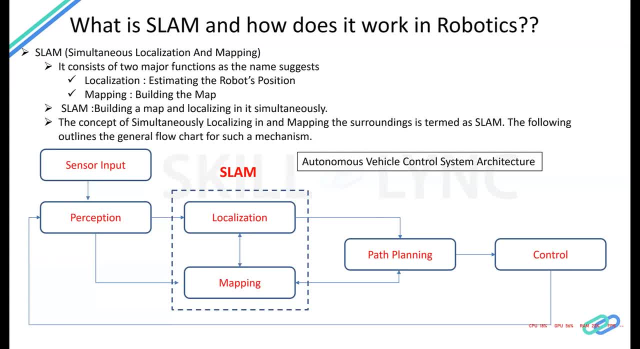 you have the sensor information right. so you need to perceive the system, or you need to. you need to perceive the environment, and then this perceived information is sent into the localization slash mapping function. what happens in localization and mapping function? your system reads the data and it will estimate exactly as to what the environment looks like in its own terms, right? so 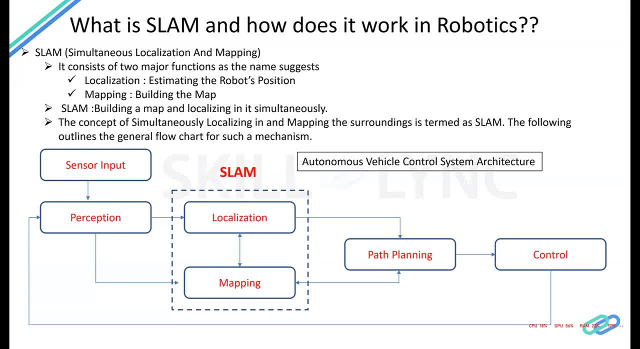 there is a number of ways to perceive the environment and we'll not go into a detail about that at this point. but so there are a number of ways to perceive the environment and now, once you have the environment and you have the sensor information that is coming in as to 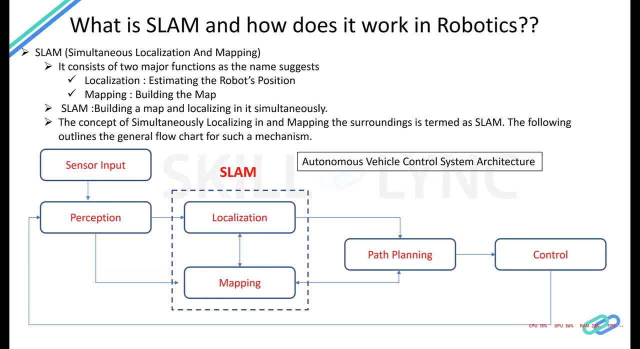 a tentative sensor information that is coming in as to where you are possibly located in the given uh map, or that is that is being read by the robot and that's where the localization function comes in. you will start to uh use this sensor information and you start to do some localization algorithm will basically take care of uh, you know putting. 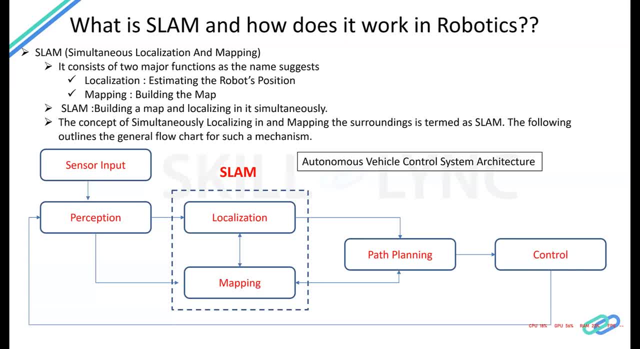 yourself or estimating your position as much accurate. uh, to the, to the maximum accuracy that it can go to. that is the main uh. that is, that is the main function of localization, and so what happens here is that the localization function comes in as well as a sensor information. it will 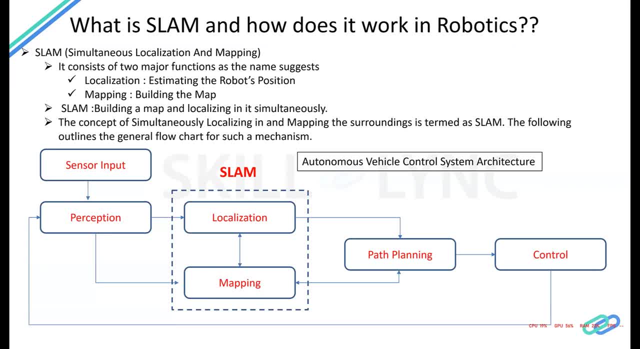 be given by a sensor. you know, persuading your data that is given by a sensor to really map the environment to the map and, of course, the most important thing is that the data that you have is available in the localization option, and the number of ways to do that is the number. 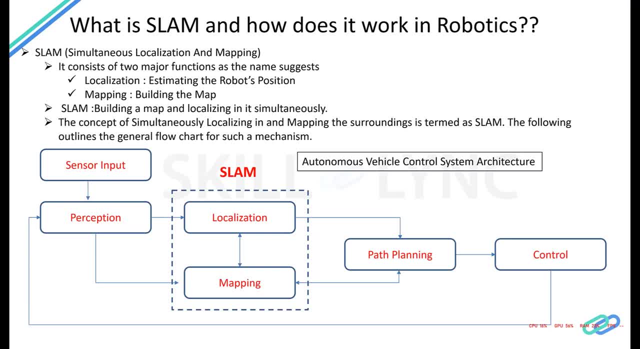 of ways that you can be on on social media or social media, and then you can actually search. for the localization and mapping done, the next step is to plan the path right for any given robot. you have a source location and a destination location, so you are trying to go to a certain 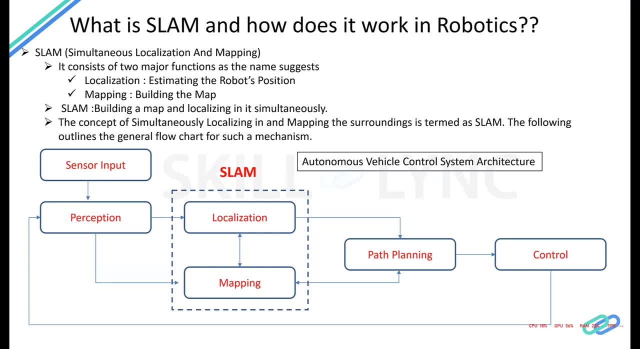 location based on the map, and you have the localized location of your robot based on the map and also the sensor input data. now you are trying to plan a path, in that you're trying to plan a path from the source to the destination. okay, um, let me show you an example for 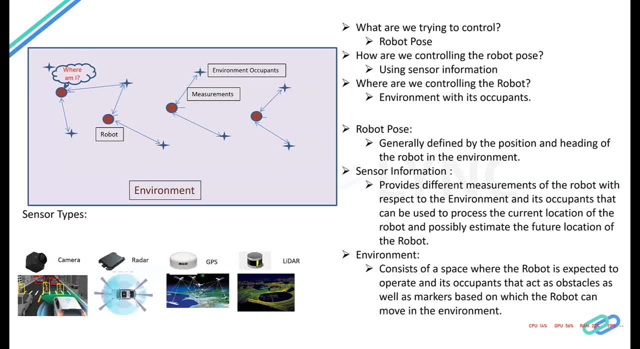 example, let's say the robot wherever it is in the first course. um, in the first course, the robot is the source it has is at its source. okay, in the last course, the robot is at its destination course. now, what are we trying to do with the slam algorithm? 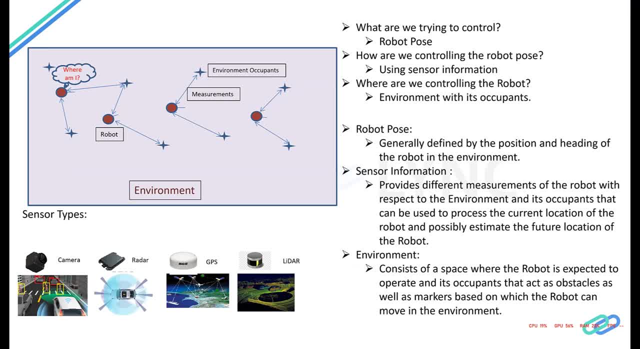 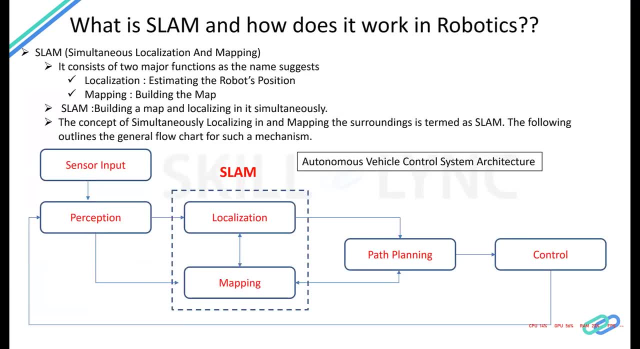 is. we are basically planning, trying to uh plan a path for the robot to go from the source to the destination point, based on the sensor information that you have available to you. okay, so that is exactly what, what is happening here in a flowchart perspective, wherein you're getting a sensor input, you're perceiving the system. 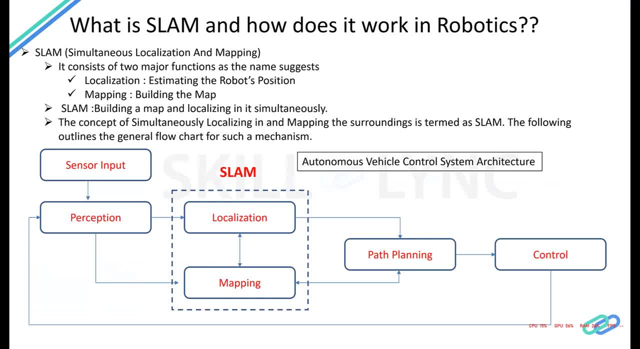 and they are perceiving the environment around you. you are performing an algorithm, you are performing a function which is nothing but the slam algorithm does um to you know, localize and map the system, uh and the environment, and then plan a path for the system to go from a source to a destination. 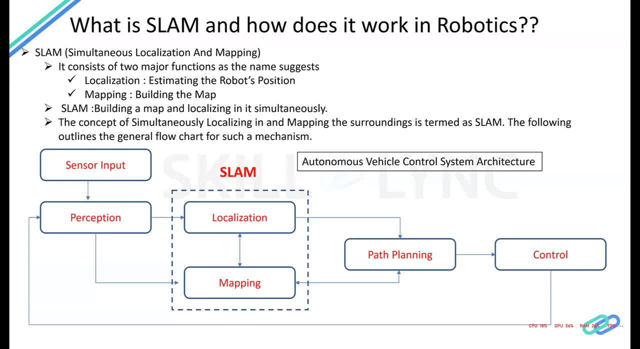 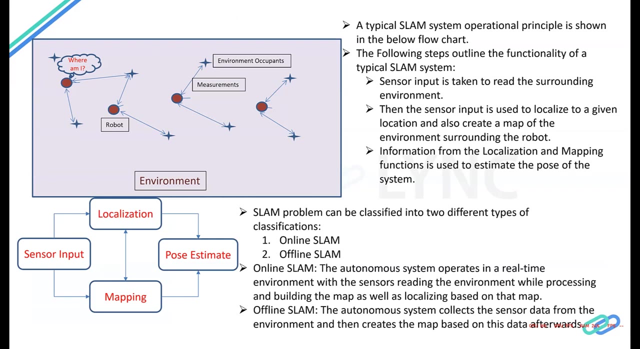 and then you generate control commands that will basically help the robot navigate in the environment. okay, so that's a very generic, uh high level introduction to what islam is. um, now moving on to the next part of this. okay, uh, as i was saying earlier, um, a typical slam system is of the. 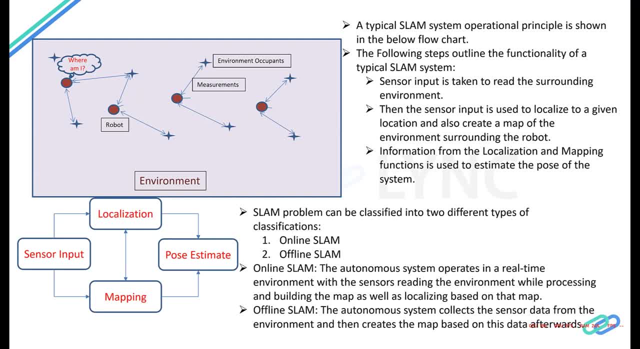 operational principle is shown as below: um. so again, i'm going to repeat the same statements that i made earlier, but hopefully this will make it more clear if it is not earlier. um okay, step one: you take the sensor input from the sensor uh surrounding environment. step two: 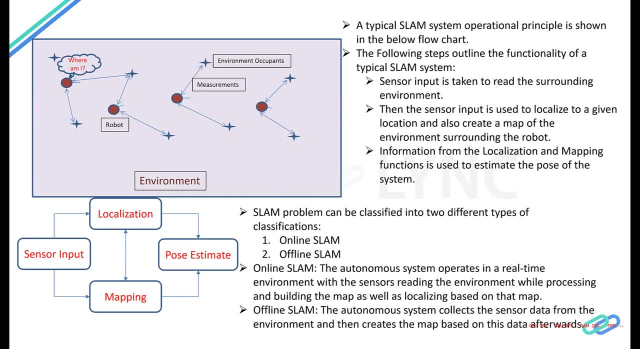 the sensor input is used to localize and map the environment around you, and this will enable the system to perceive itself as to where it, where it is on the or it will give it, it will give a. um, let me put it this way, the localizer, the sensor input, will. 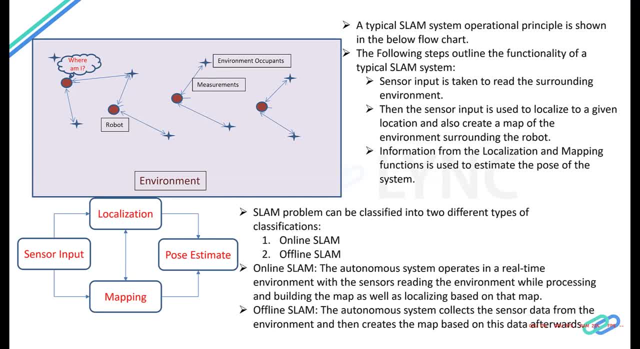 give an information as to probably possibly where can the robot be in the given environment, and it will simultaneously construct the map of their environment around the robot. okay, so now you have the map that is constructed around yourself and the localization functioning that is trying to estimate the best possible position of the robot. 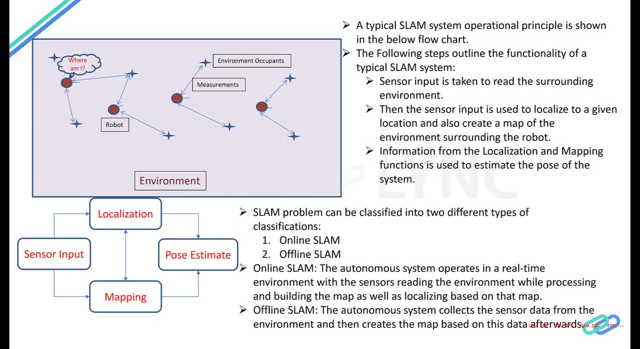 and that function is done by the slam algorithm. okay, so, as you can see, um, this is a simplified- uh, the bottom picture, the bottom flow chart, is a simplified, simplified version of localization and mapping algorithm. um, so, basically, you have a sensor input, you are taking it into localization. 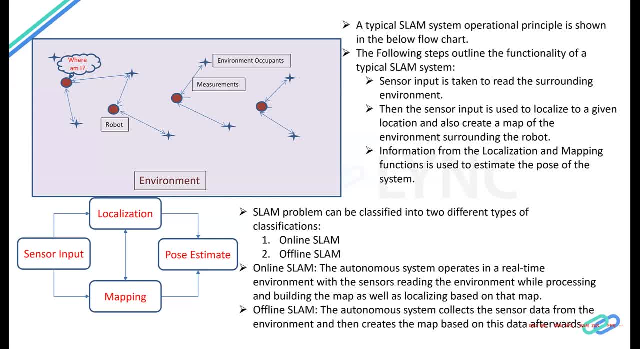 mapping functions. it can be one function, it can be two functions. there is a lot of ways to design it. um, and you're using the sensor information to localize and map the map, the environment. localize the system and map the environment and then estimate the pose of the system based on. 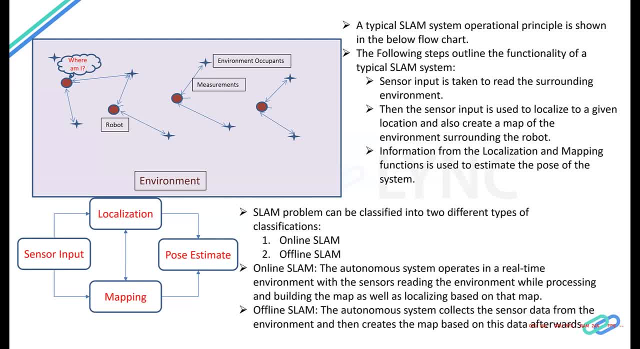 these two inputs, or these two, the output coming from the localization mapping functions. okay, let's stop. let's talk about, uh, the how the slam functions are classified. as to us, um, as it is today, um, there's two ways that you can classify a slam problem: one is online and one is offline slam. 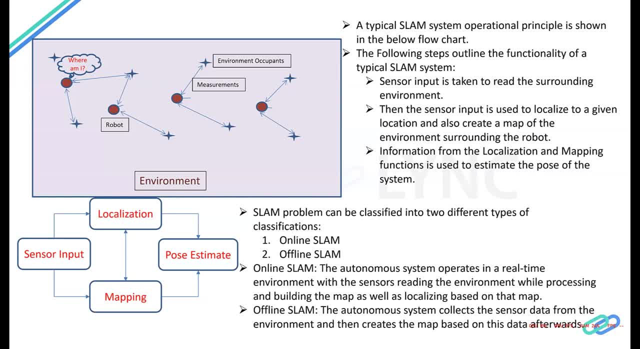 um, online system are basically, uh, real-time- uh, they work on in real-time environment, wherein, um, your sensors are reading the environment and also localizing the vehicle or the robot that you're trying to localize onto the map simultaneously, which means that, um, your system is reading the environment. 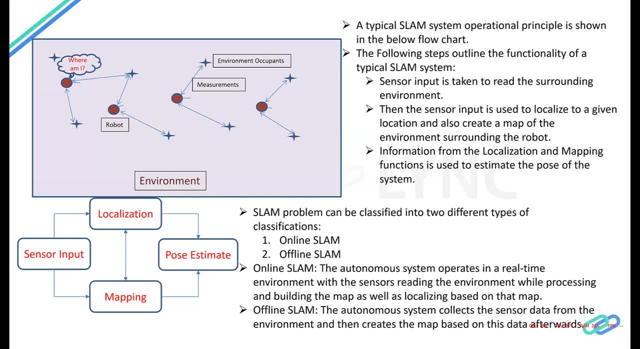 and processing the data to localize itself onto the, onto that- uh, you know- map of the environment, uh, in a simultaneous fashion. okay, um, the second different, the second classification of this is going to be, uh, offline slam. offline slam is a type of system that is going to be like a kind of like a. 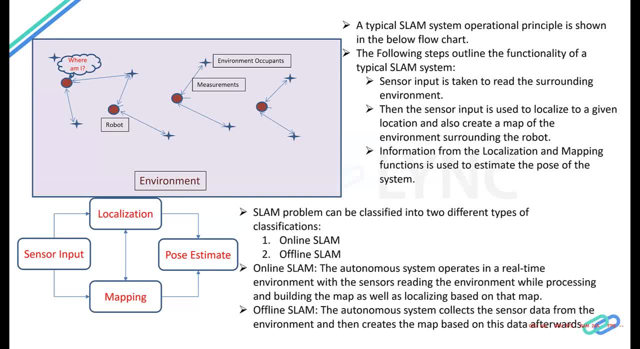 is nothing, but it collects the data of the environment in a before and then the map and then creates a map for it and this map is used to localize robot. you know, let's the in a different way or after the map has been constructed, using this previously collected map information from the sensor data. okay, 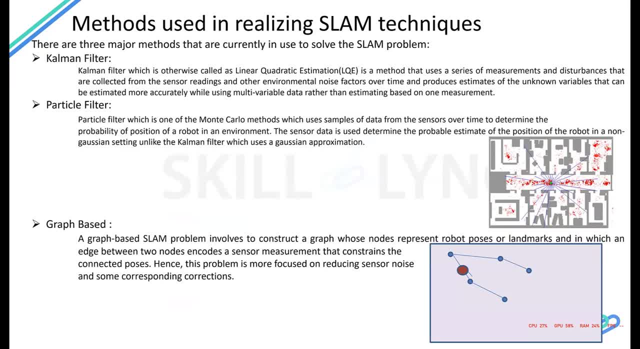 going to the next one. okay, here are some of the examples, or here are some of the methods that that are currently in use for different slam systems. okay, a slam, okay for any- let's talk about generic system. okay, you have many different methods of like you can have an, you can. 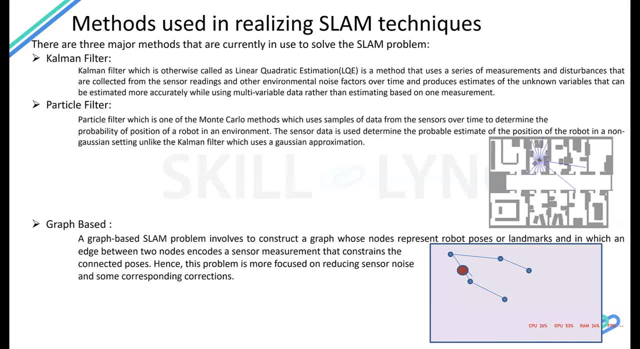 have a number of methods of doing or realizing a certain function, right, so what? what are the different methods of, you know, realizing an algorithm? here are. here is here are three examples. there are many more methods that are that are used on a regular basis, but here are a few. 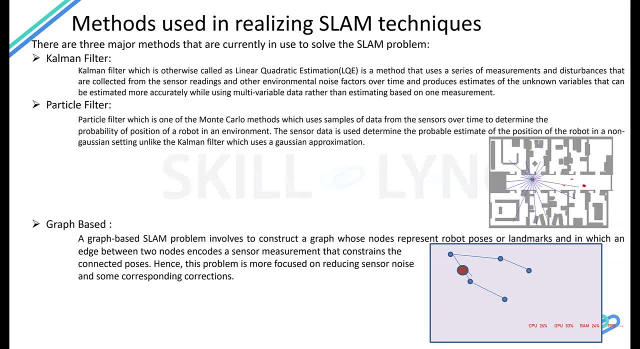 a, a, a good examples as to the methods that are used in this in resolving the slam problem. okay, the first one is a Kalman filter. what is the Kalman filter? here I'll give you a very high level introduction. we can go into details once. 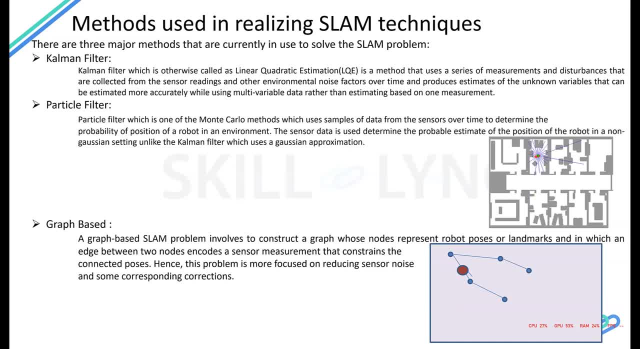 we have started up to the course, but here we'll give, we'll talk about these different methods in a very brief fashion. that way you get a flavor of what, what kind of you know how are you approaching the problem and how are you solving it right? so this is a slam problem is nothing, but it's a. 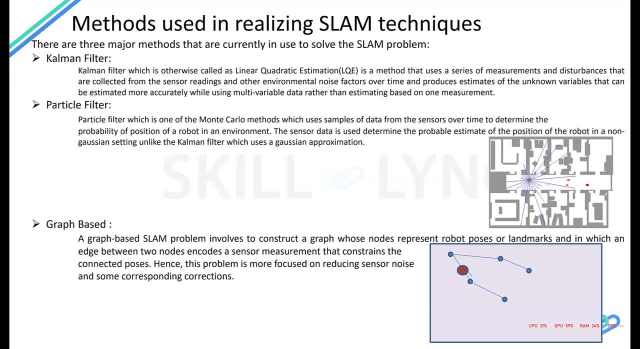 mathematical problem, right? so you're trying to solve a mathematical problem wherein you have- so let me put it this way, you have- the sensor information, right? so how do you? the mathematics is called the universal language because in this case, you're trying to read the environment, right? how do you read the? 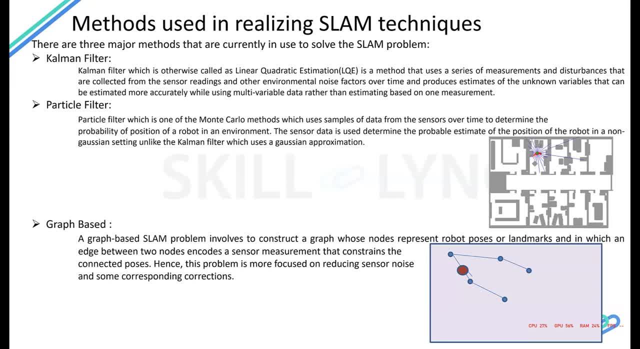 environment based on certain measurements, which is nothing, but it is converting into some kind of you know where, something that will involve some, some level of mathematics to it. so these different methods of you know solving a thought slam problem, they will help us perceive this mathematical problem and 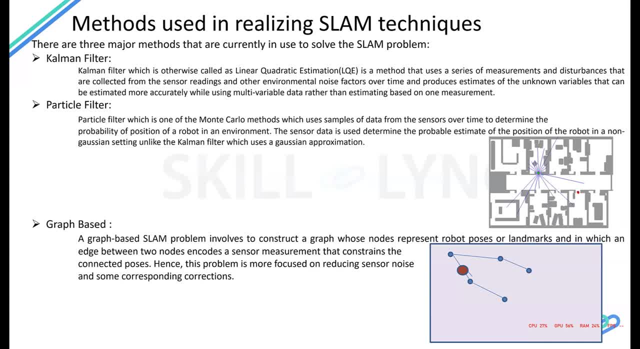 solve it right. so that's the first one, and then the second one is, you know, the five number part. that's the step you have to do and that will be used as an allotment, and then you have the bachelor of the math system and that is exactly. 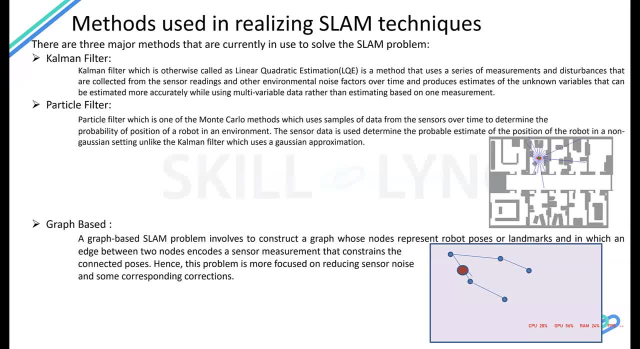 what is happening here. let me talk about these different functions in a very briefly, and then we'll go ahead and, you know, talk about some more advanced functions as well in the next couple of slides. so, Kalman filter: okay, I'm going to give you a very brief introduction of these. 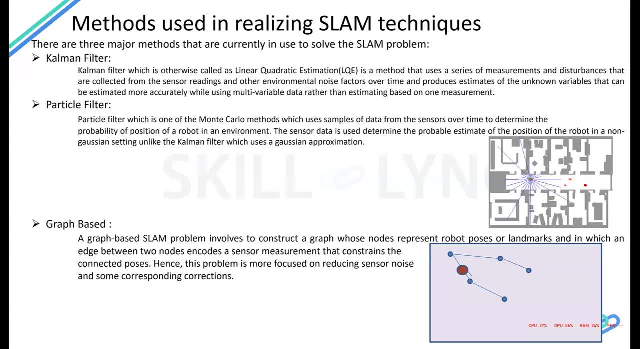 methods that uses a series of measurements and estimates from the environment and produces the estimate of the unknown variables that can be estimated more accurately while using multivariable data. This might all seem to be a little bit new to all of you, but let me help you understand. 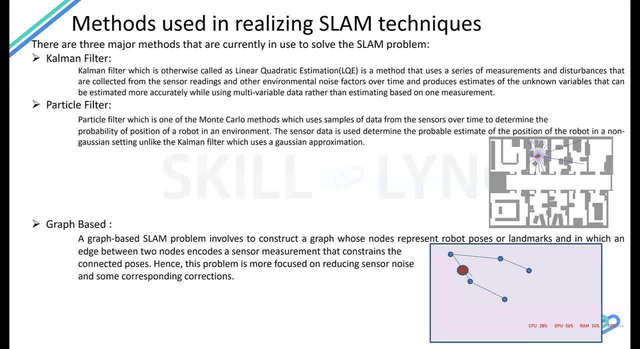 this. Okay, so let's say you have a robot, right, So you have a robot. What are you trying to perceive for the robot? One distance from any given environment, right, That is one. And then position of that or heading with respect to the environment. 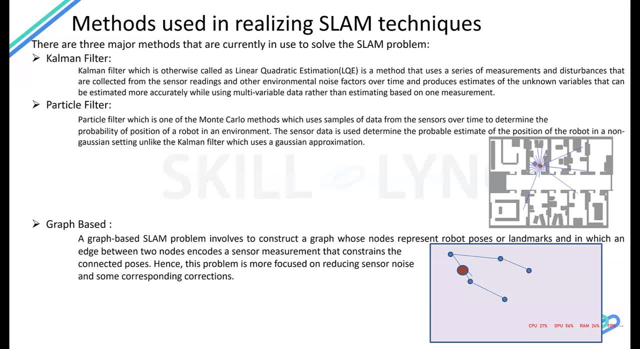 With respect to that particular orientation of you know, the object with respect to the robot or the robot with respect to the object right. All of these come down to certain mathematical numbers, one of which is going to be distance and one of which is going to be heading. 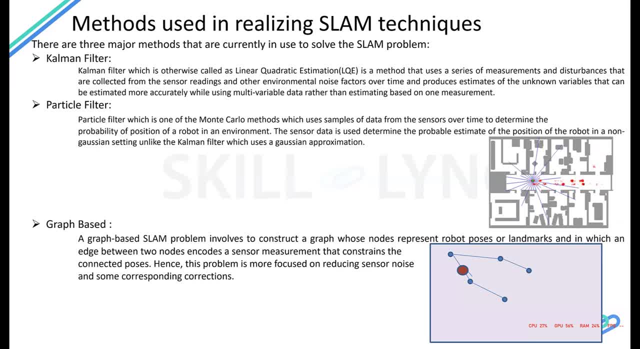 You can, let's say, let's say we're talking about the green dot that is shown in the bar in the bottom picture, the picture in the middle. So what is it trying to do? It is trying to take measurements, right. 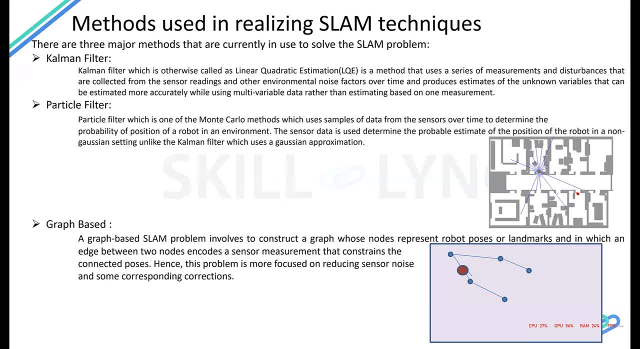 It's trying to take measurements and it is trying to map the environment as well, as you know, estimate its position based on the information that it has available. So the information that it has available is represented by the blue lines down there. What does those blue lines represent? 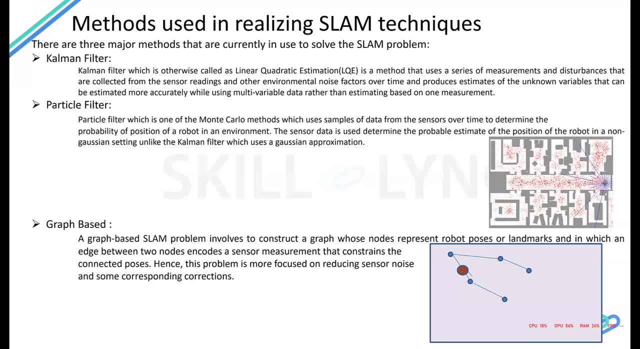 One distance, Second distance, Third distance And finally, the third is the heading: with respect to heading of the object that it is the robot is perceiving with respect to the robot right. So these two information will be the sensor information that the robot is taking in right. 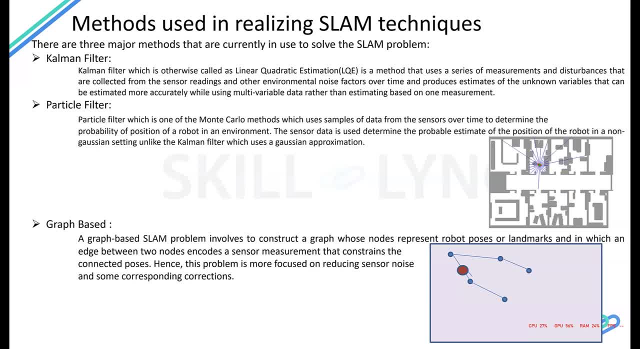 So in this case you let's, because we are talking about the Kalman filter. let's take that example. And you're trying to apply a Kalman filter on the green dot Next given on the picture below, and you know the green dot is your robot and you have the surroundings. 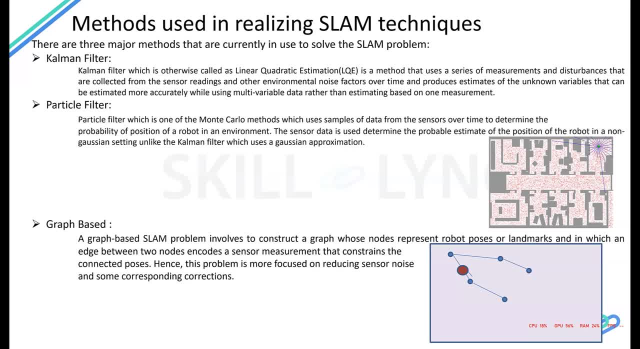 around you. so you are trying to produce estimates for the unknown variables. what are your unknown variables? your unknown variables are going to be your position and your unknown variables are going to be your position. and you know the heading of the object or the robot right. so now we know what we need from the robot right. what you need is your position. 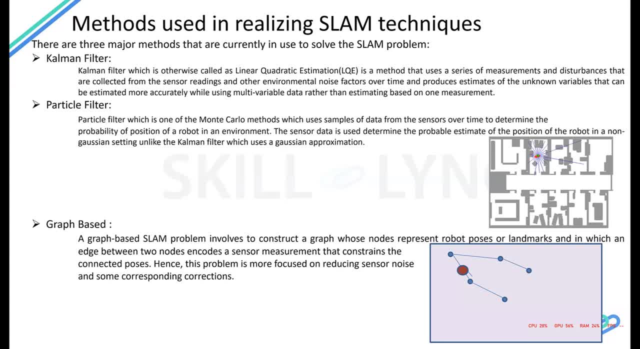 and your heading of the robot. now, what do we know if your position is untouched or not? any maid, whatever is the sensor input that you're getting from the environment. what do we need to work with the work? what do we need to do? so, if you might have had a, 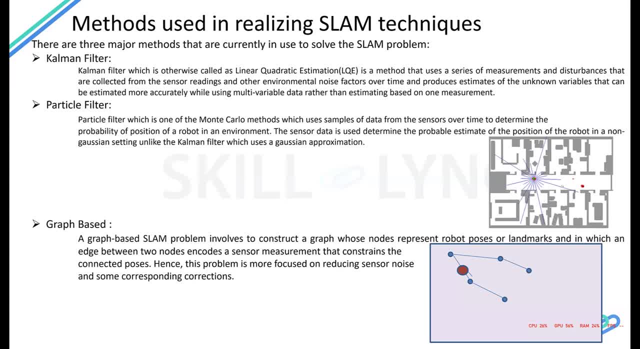 background with control systems, you would understand that any given system or any given object in the environment, in any environment, can be perceived as a mathematical model. the mathematical model is nothing, but it represents the system state, which means that any given system can be represented in a you know. 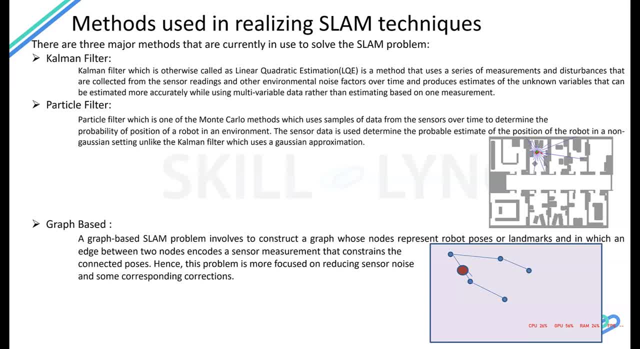 in a mathematical model and this. but this mathematical model can be estimated based on the sensor readings and you know all the other inputs that are that can be used to generate the mathematical models of it. so you have, so you have the sensor reading, and then you have the sensor reading and then you have the. 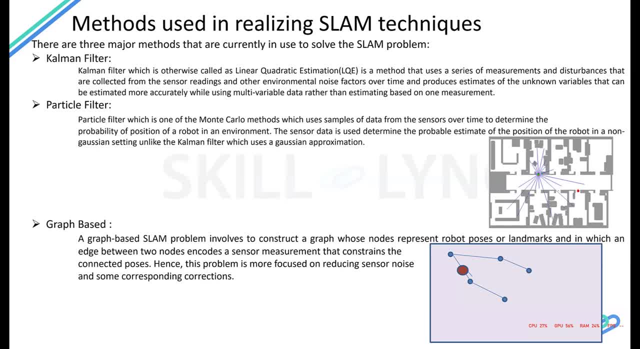 certain estimate of the certain model that you're trying to generate for the system. right, so there is a predefined. so, generally, what happens is you have a predefined structure for the you know system, the way it should be, the way it should be modeled, and then you try to estimate the different variables that 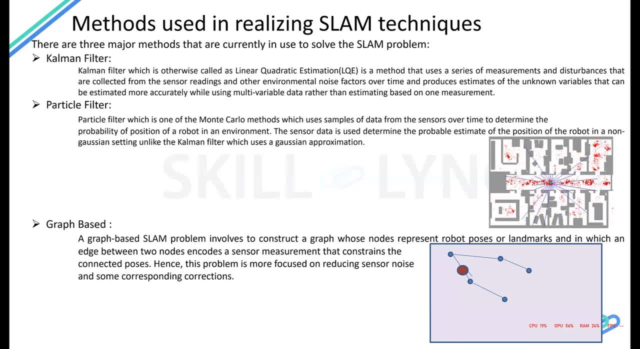 you have in that system, based on the information that you're getting from the sensors, and then you try to, you know, tune it as you go. that way you get the correct mathematical model that represents that system. okay, let's take an example: helicopter. you, if you are, if 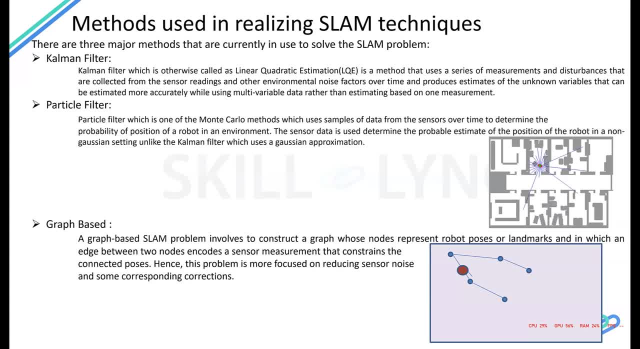 you are in from one of this background, you might know this. you might perceive this better, so I'm going to. so this is a very generic example, so I'm going to take that example to explain the attributes of the system that will define it. which role you are define will define the orientation of the vehicle. 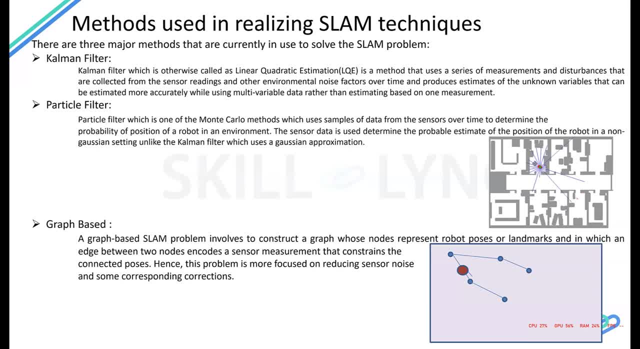 and then the vehicle velocity, along with this bit solia and all these different system system variables will define as to where the vehicle is and where it is going to, and all of these different factors. so now, in order for you to do this, you need to have certain measurements taken from the environment. 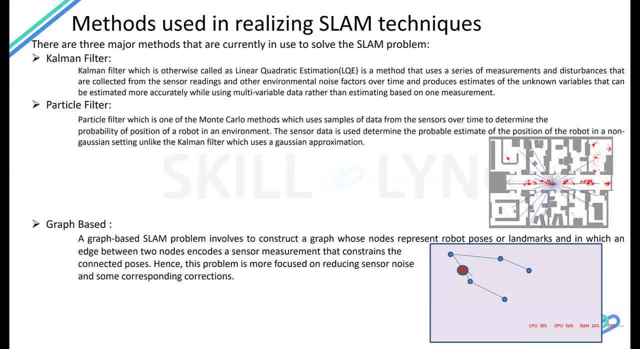 you're taking it from different in one. sensors can be GPS, it can be a camera sensor, it can be whatever it may do. you have the input for the system, or you have the input for the system to be sensor input, and then you have a certain system, which is the structure of which is: 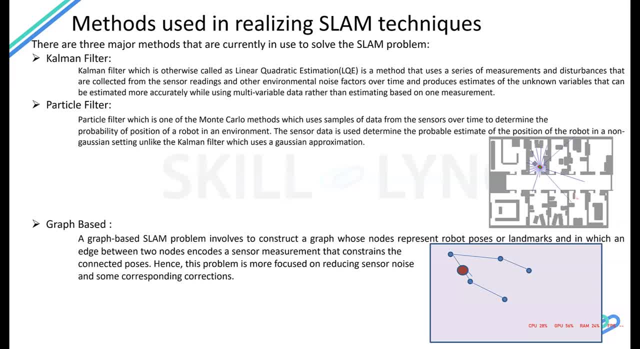 predefined to some and you start with it and then you have the sensor input and then you try to. you know, use the sensor input to reduce the errors and you know the noise sector that is coming from, the environmental factors and estimate system, mathematical model, and try to correct it over time. so that is exactly. 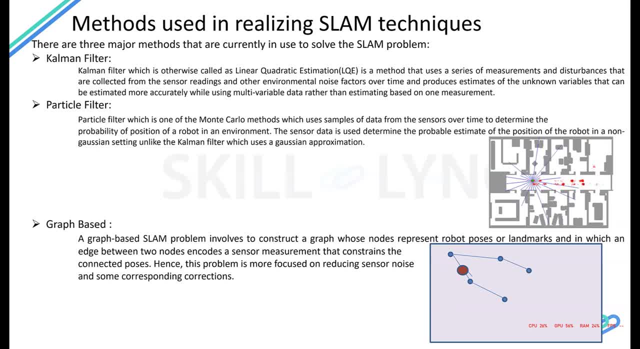 what happens? the norm Kalman filter. okay, so you're basing your estimate of of the system or on a given mathematical model and you're trying to get the best out of what you can, to you know, represent the system in the environment. hopefully that's clear. moving on to the particle, 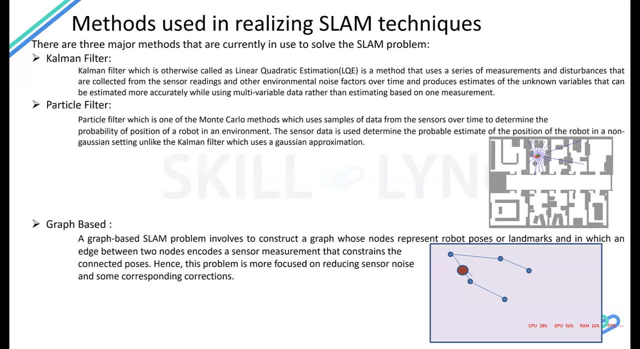 filter. particle filter is nothing, but it's a probabilistic problem. when you start the robot in a given environment, then it will think that it is all over the place. it can be anywhere within the entire room. right now, what happens is as you go around, as the robot moves around the environment. 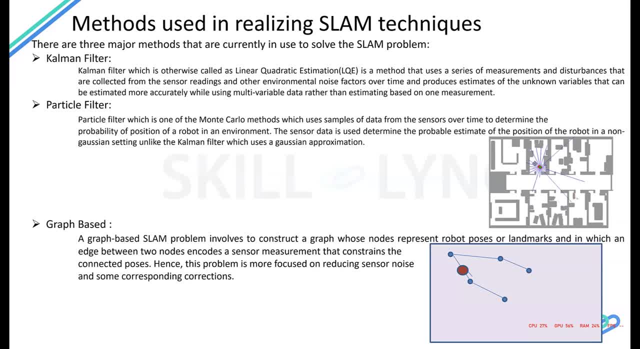 start to map the you know environment and it will start to generate the probability of it being at a given location. as you move around and as the calculations regarding the probability of a given position based on the sensor input are going on in the background, you would see that the probability 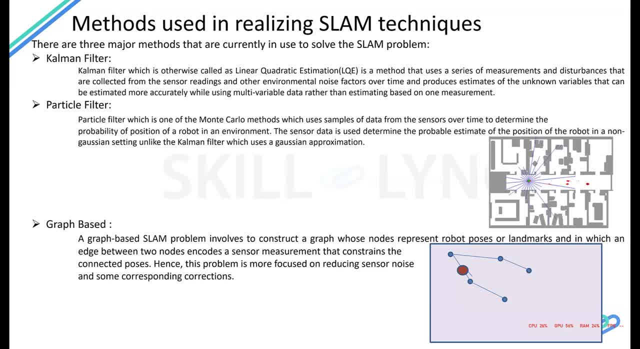 will slowly come down to. you know very confined certain location. it is not perfect but it is as accurate as you can get you know with with the sensor input that you have. so it depends upon a lot of factors as to how accurate can you get with the system. but probabilistic method. 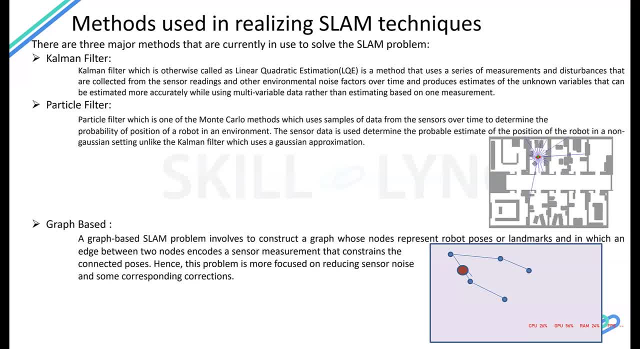 wherein you perceive the environment and then you know, you read the environment and you generate the probabilistic position of the robot based on this sensor input. that that basically defines higher level of particle filter. now, coming to the graph based method can be an example of, before i go to. 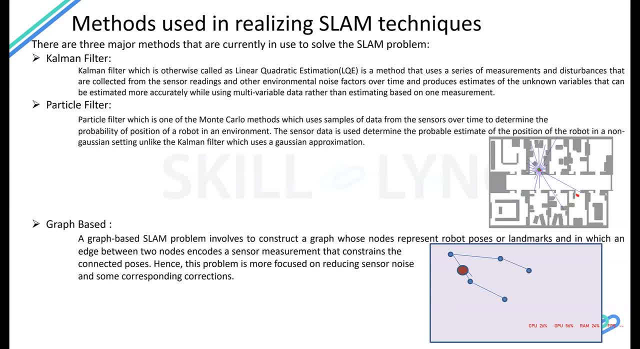 the graph, we were talking about the online and offline slam methods, so kalman filter and particle filters can be considered as one of the two of the online methods wherein you are doing the mapping and localization simultaneously, and these are two different methods that you can do that, okay. 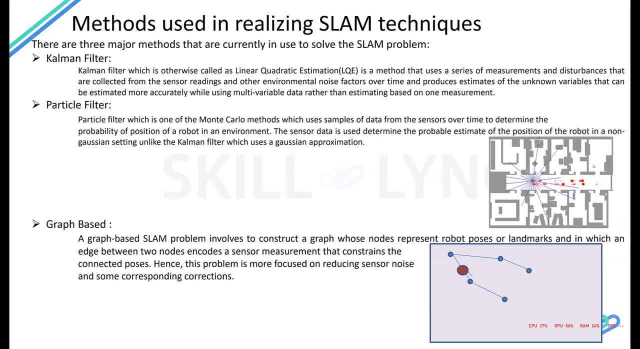 now graph method. graph method can be considered as an offline slam method. what is an assurance? last night slam method, like we discussed earlier you have, you generate a map based on the sensor input and you use that to at a later state to localize yourself onto the map. 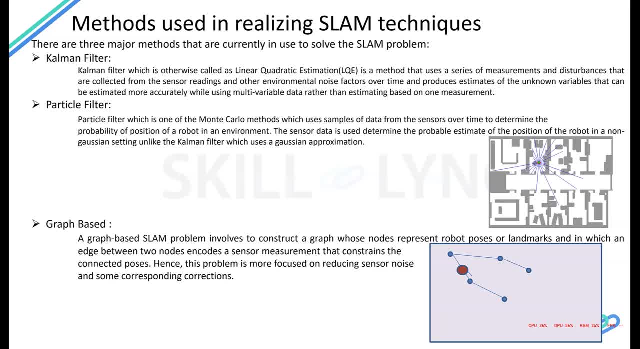 that's what is happening here. so your graph network will define, will represent the environment on the map which are predefined and your robot robot will localize to these, to this map on the graph network, to show exactly where you are at and you know your location and, of course, all the other, um, all the other characteristics of the robot. okay, so now. 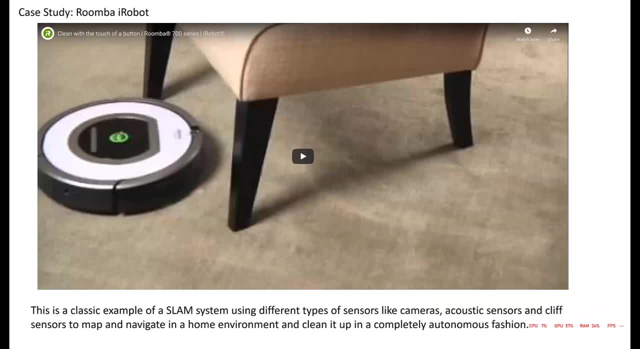 going on to the next one here, i'm going to just play this video. just have a look at it. um, this is a very, very familiar example as to where the slam example, slam robotics or the slam methods are used in a very expensive way. um, i'll leave you to listen to this for a second. here the robot automatically. 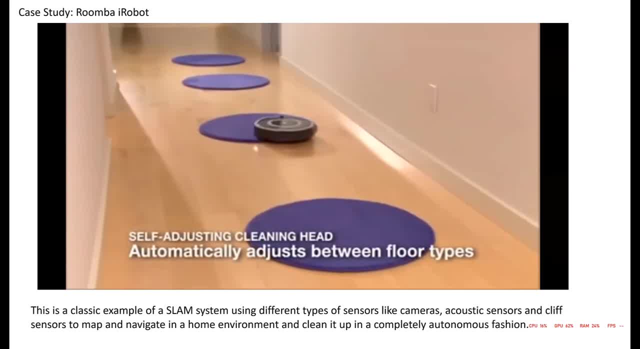 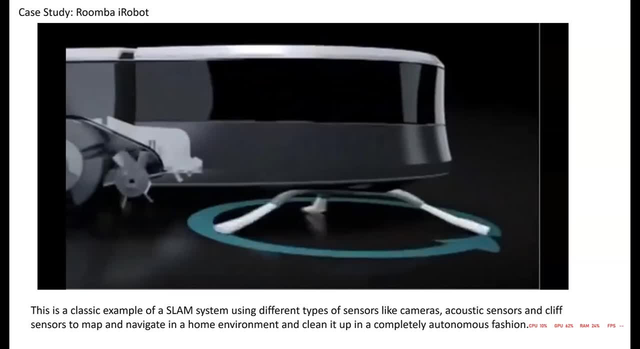 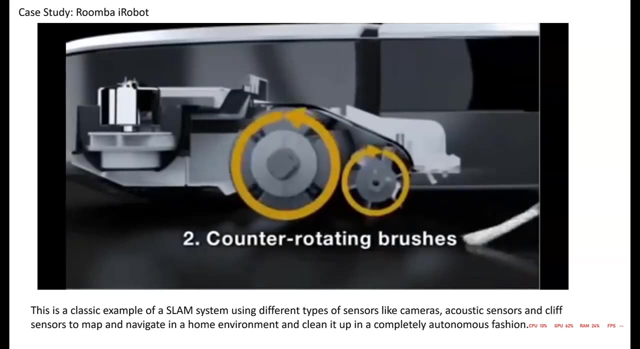 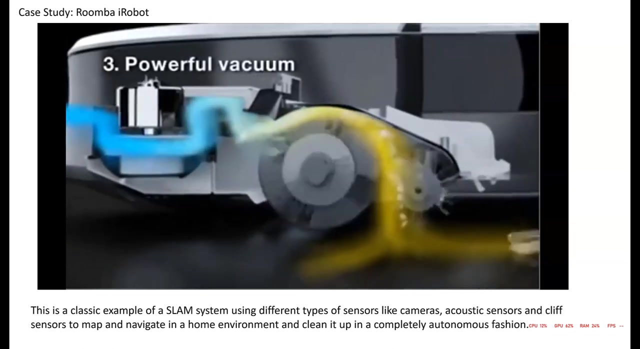 self-adjusts to different floor services as it moves through your own roomless. patented three stage cleaning system provides comprehensive cleaning coverage. first, the spinning side brush cleans along wall edges. next, two counter rotating brushes scoop up dirt and debris. Finally, a powerful vacuum folds it all into the bin where the filter cracks dust and other fine particles. 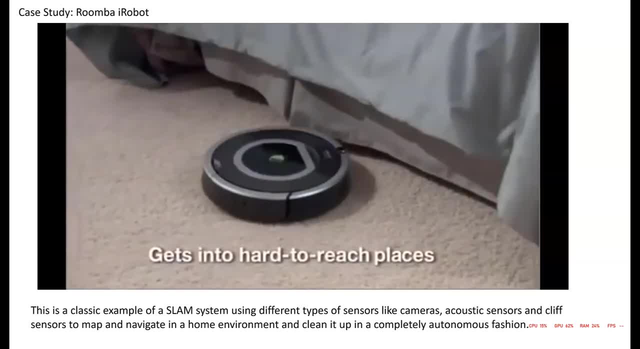 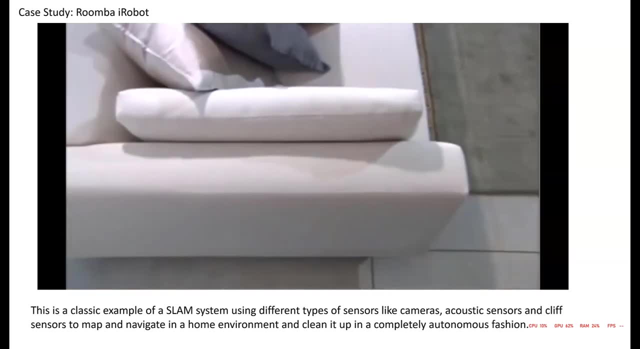 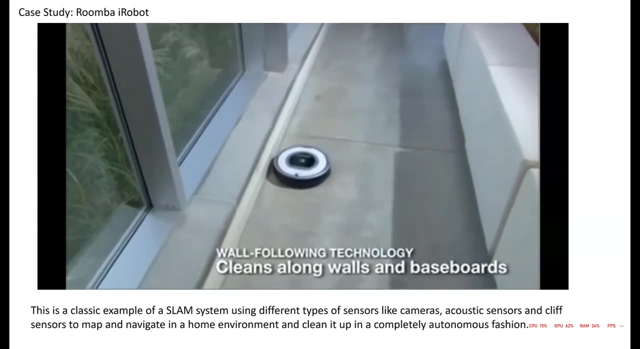 Roomba cleans under the bed and other hard-to-reach areas. Unlike an old-fashioned upright vacuum, Roomba cleans in tight spots and under and around furniture. Plus, Roomba uses wall-following technology to clean along walls and base floors and ensure the whole floor is completely clean. 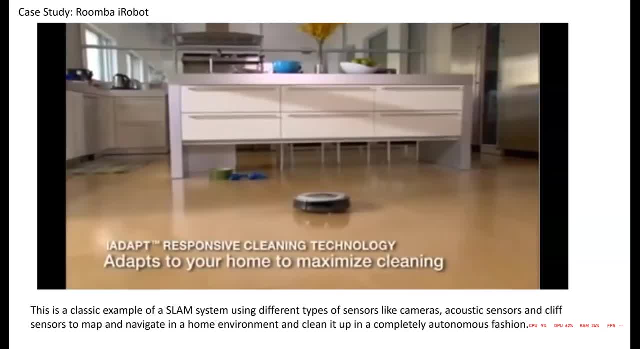 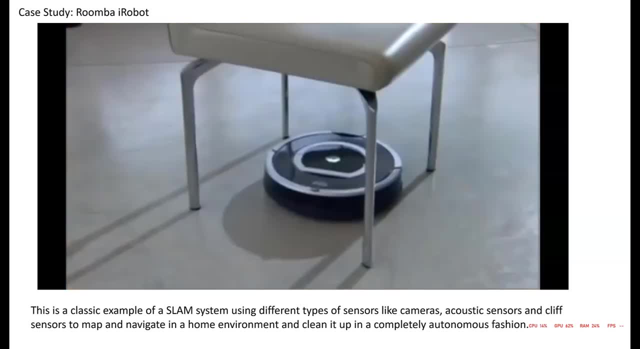 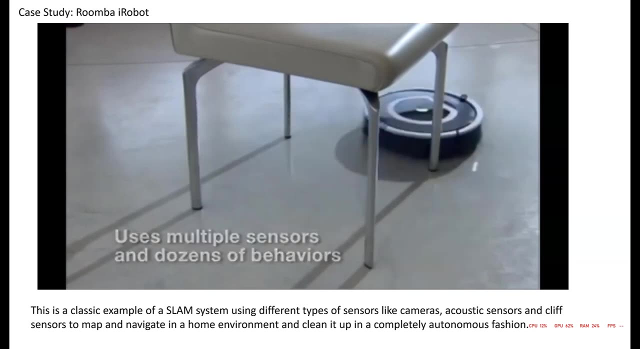 Roomba maximizes cleaning by adapting to your unique household environment. Roomba's iAdapt responsive cleaning technology monitors the environment more than 60 pounds per second, using multiple sensors and dozens of behaviors to clean your home. Roomba's soft-touch bumper provides a cushion to clean your home. 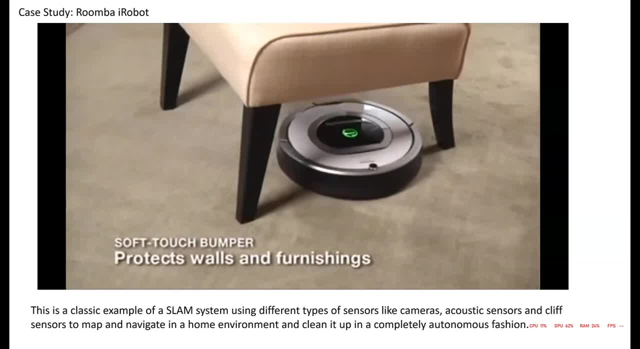 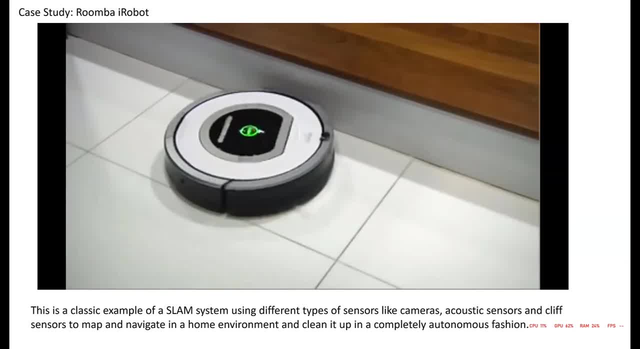 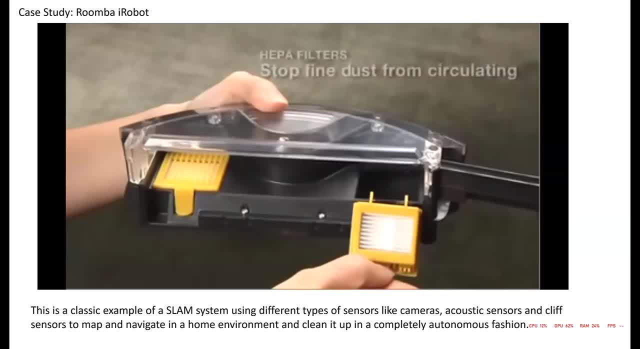 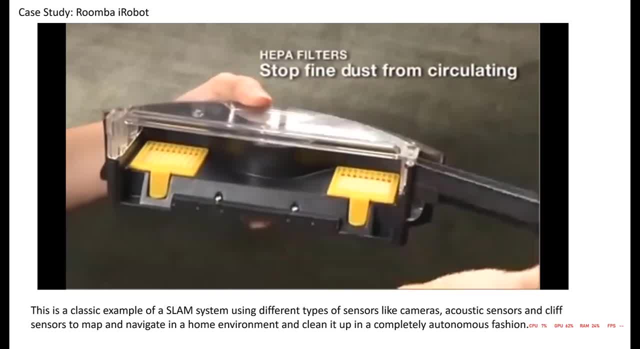 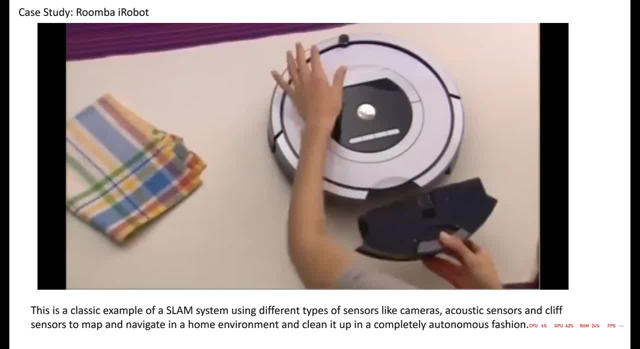 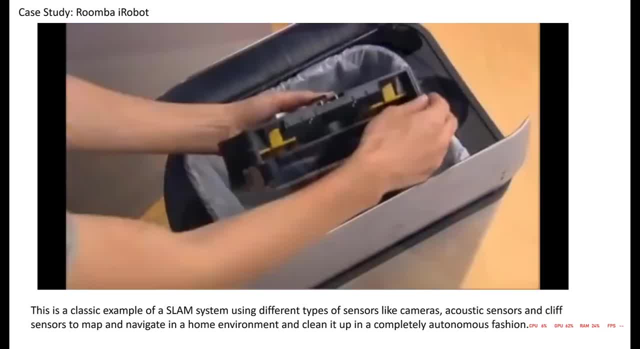 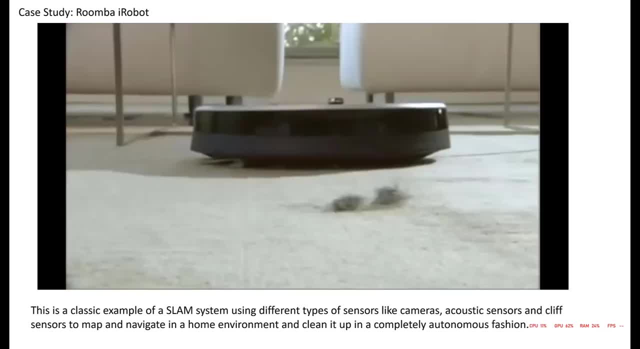 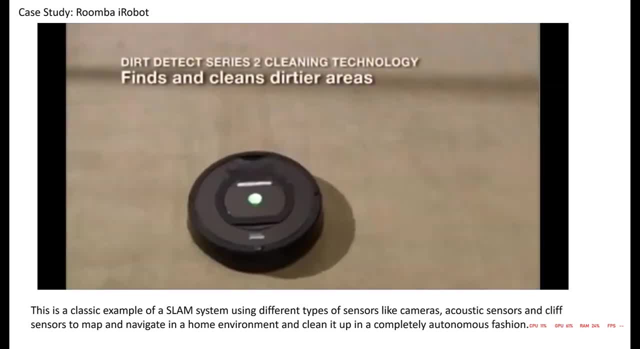 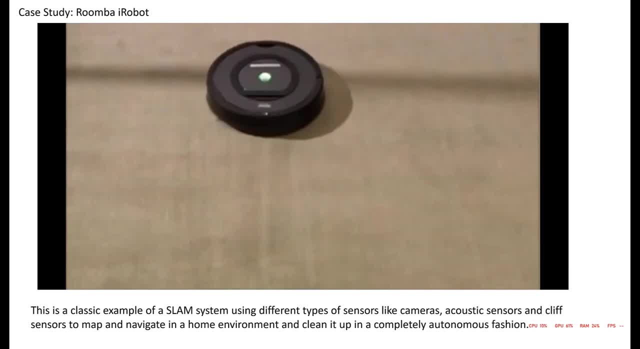 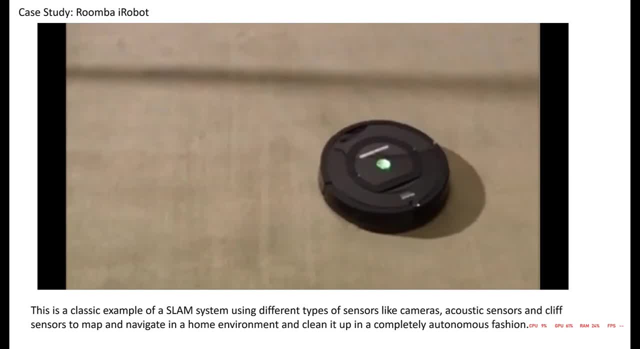 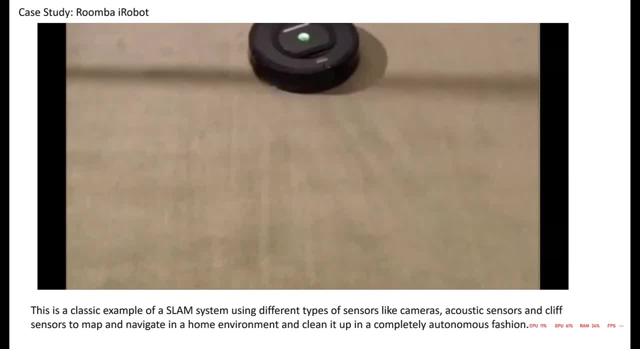 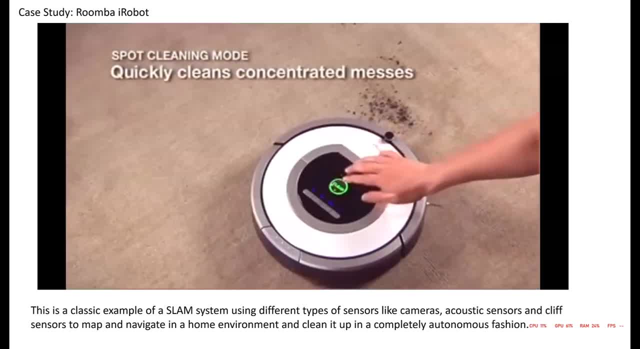 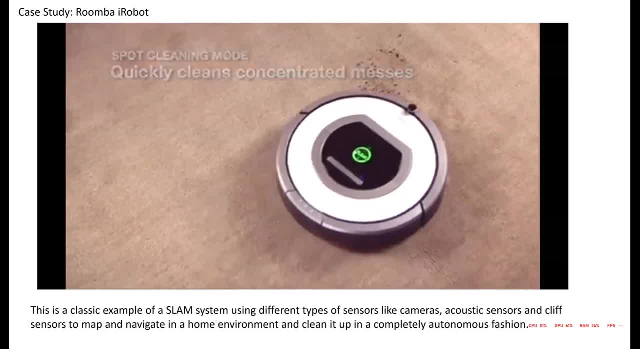 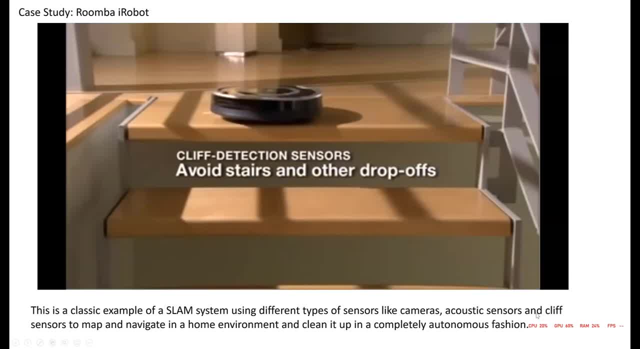 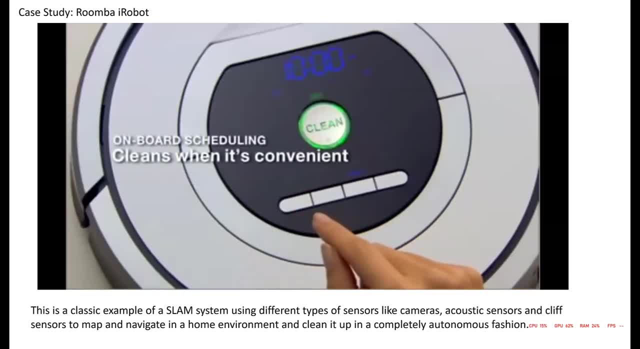 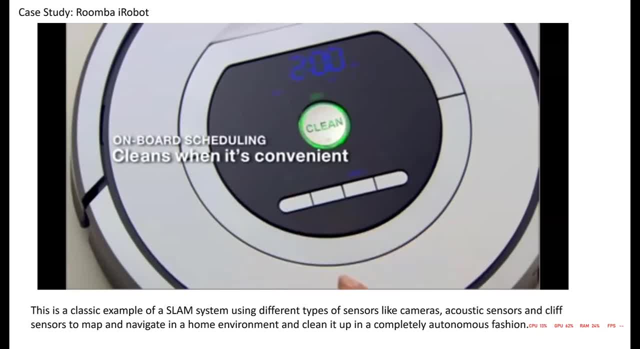 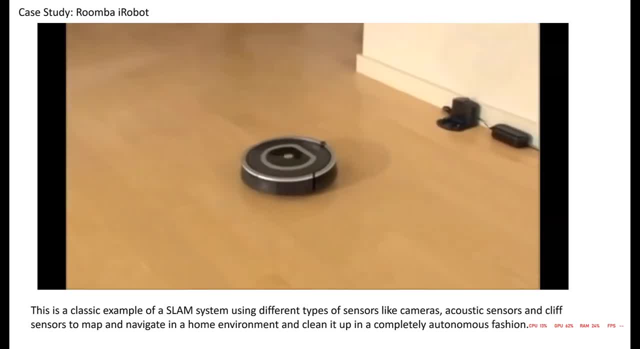 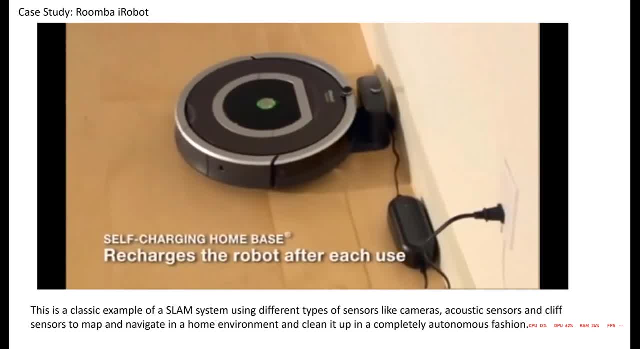 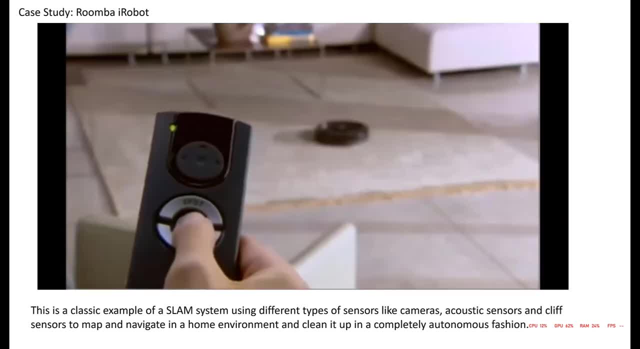 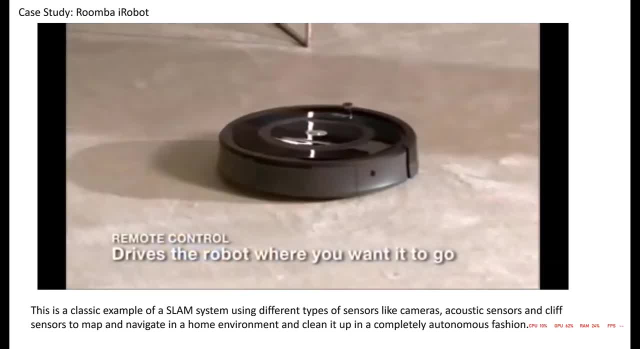 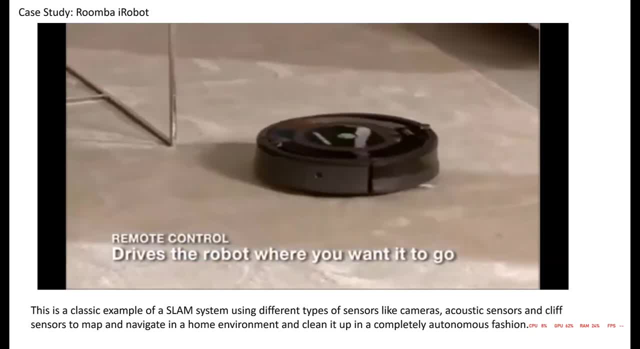 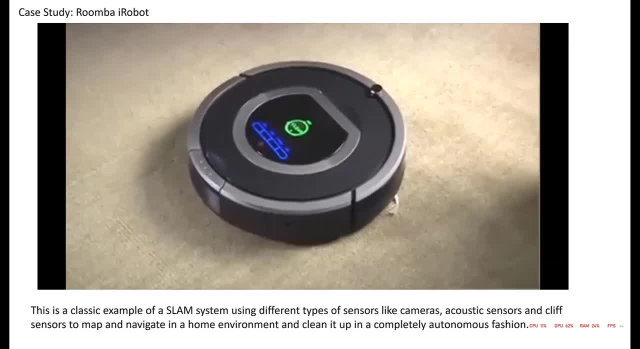 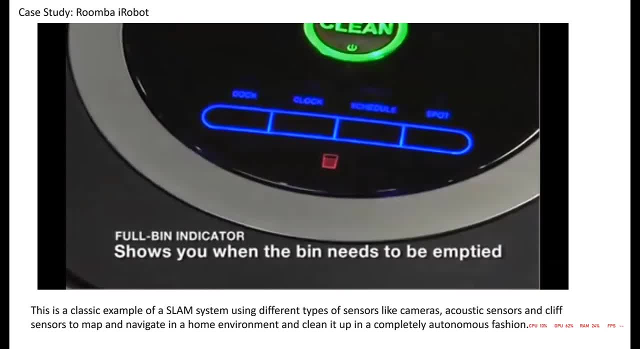 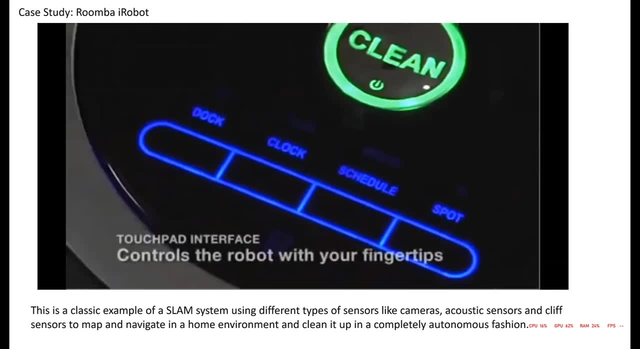 Roomba's soft-touch bumper provides a cushion to clean your home, an indicator light to let you know that it needs to be answered. Roomba is so easy to use. The robot's intuitive touchpad interface eliminates mechanical buttons, letting you schedule and. 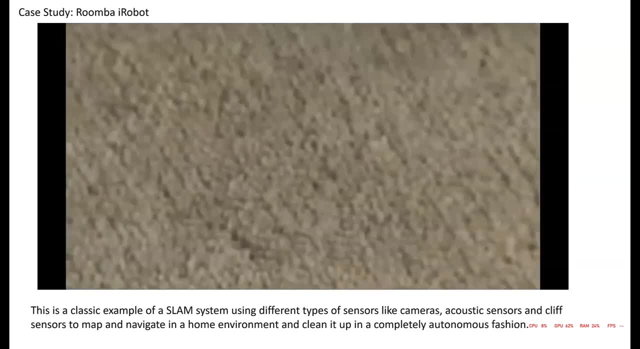 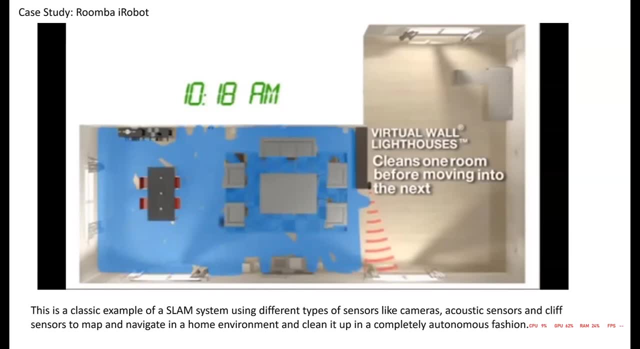 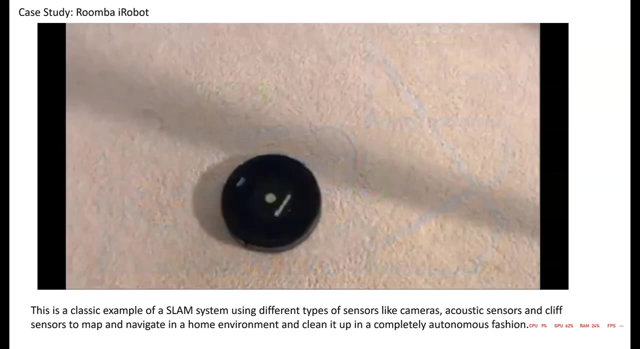 control the robot with just the touch of your fingertips. Roomba methodically and thoroughly cleans multiple rooms. Virtual wall white houses ensure the robot can fully clean the entire floor in one room before letting it move into the next room. The iRobot Roomba vacuum cleaning robot. 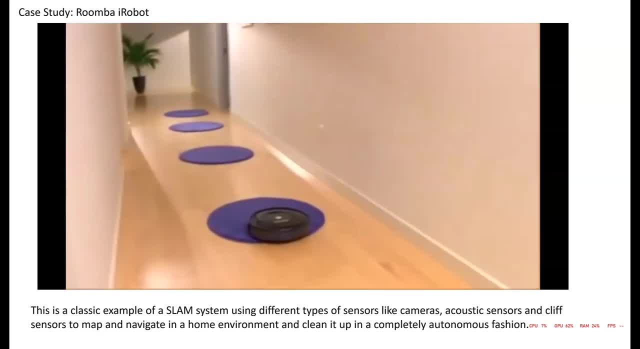 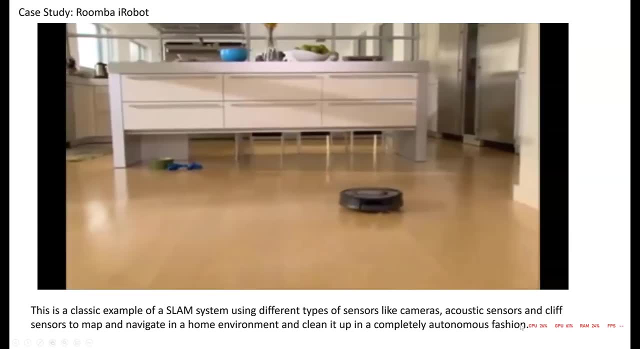 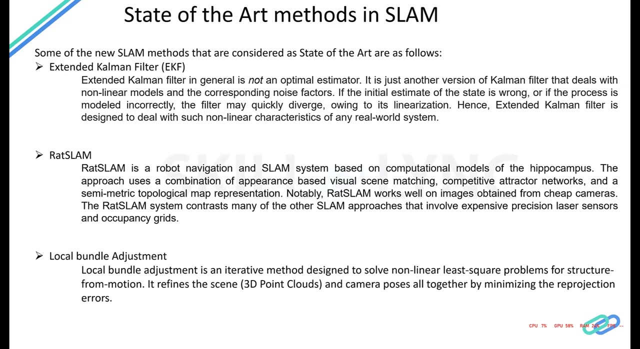 cleans your carpets and floors on its own, so you don't have to Just press the clean button and let the robot do the dirty work. Now, coming to the state of their technology. in SLAM there's a lot of I mean. in these days, technology moves very fast and you won't even know that you. 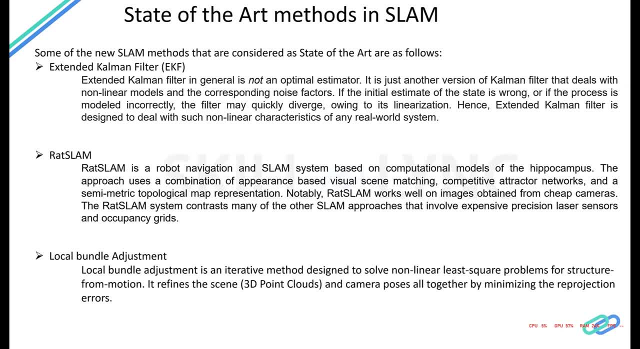 have a new method to you know, resolve a certain, or on your new approach to a given problem Before it, even you know, comes into the market. So there's a lot of advancements that are going on in this regard, but we'll talk about. we'll talk very briefly about three methods that I thought. 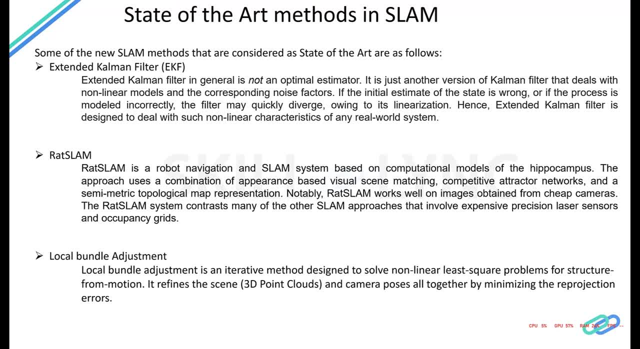 were really interesting, So one of which. let's start with the extended Kanban filter. Okay, So, as I was already talking about the Kanban filter earlier, but extended Kanban filter is nothing, but it defines the system in a mathematical model, And then you use the mathematical, you use the sensor. 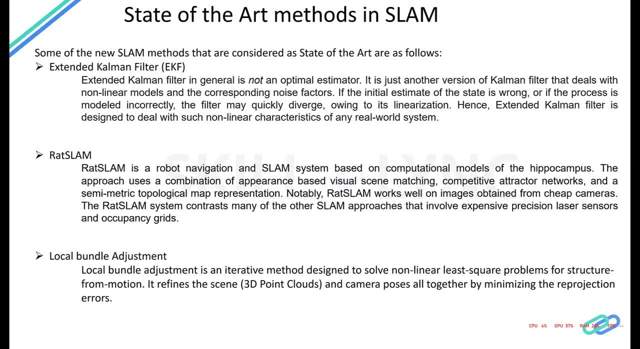 information to correct yourself and use, generate a good model of the mathematical model of the system and then use the sensor input to localize and map the system based on this information Right. So extended Kanban filter is nothing, but it also. it also enables us to you know, generate, 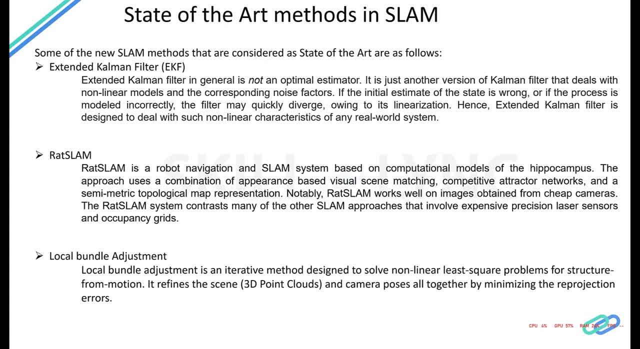 the same model and also map and localize Even though there are non. there is non-linearity present in the system, right? So any given real system is a non-linear system in general. How good you are able to linearize the system and how good 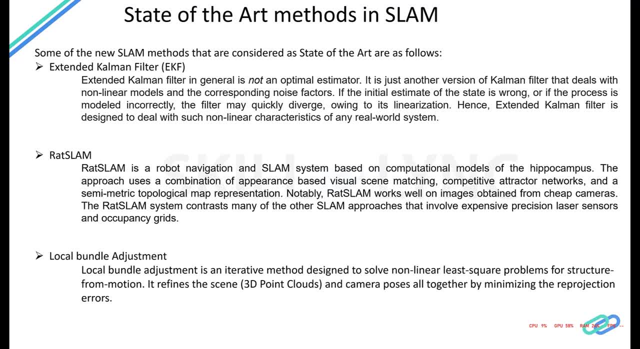 you are able to, you know, use the system to generate a good model out of it. That's what the extended Kanban is. what is the goal at the end of the day. So extended Kanban filter is nothing, but it is an extension of the Kanban filter. 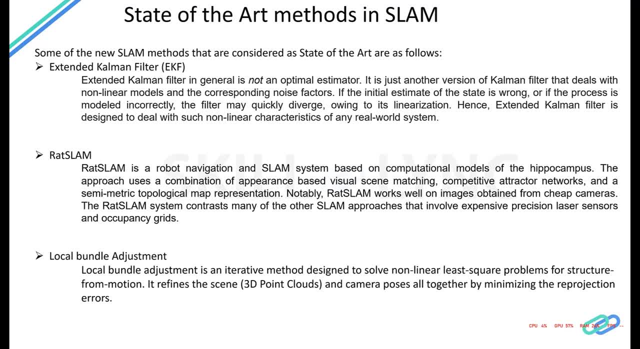 With the ability to, you know, deal with non-linear characteristics that are generally expected in any real world system. So that's a very high level detail about that. Coming to RATSLAM, RATSLAM is nothing but it's a method that is based on the, you know, hippocampus, hippocampal model of the rat. There's a lot of 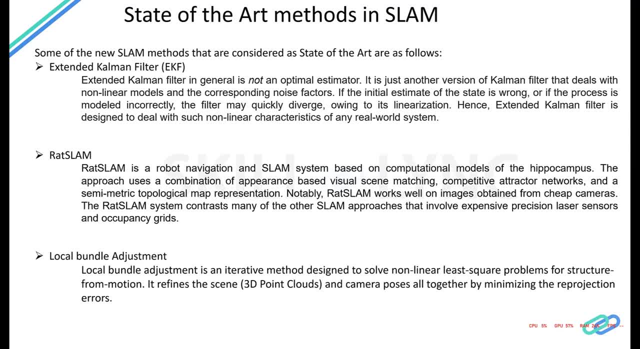 visits. that happens, that is happening today based on, you know, the neural networks and all of these different new methods that are coming into play today. So this one RATSLAM is nothing but it's a system model. itself is based on how the rats are able to perceive the system, and you know. 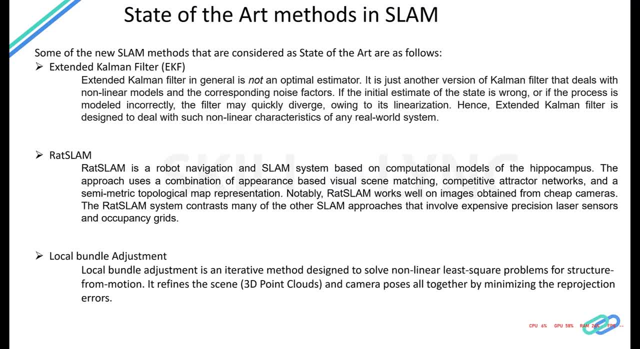 place themselves in a given system and all of these different information and how it is perceiving information and how it is processing information. So that model is being used to develop an algorithm to do that. Now, coming to the local adjustment, local bundle adjustment, this is a visual method. It uses a visual method to you know. 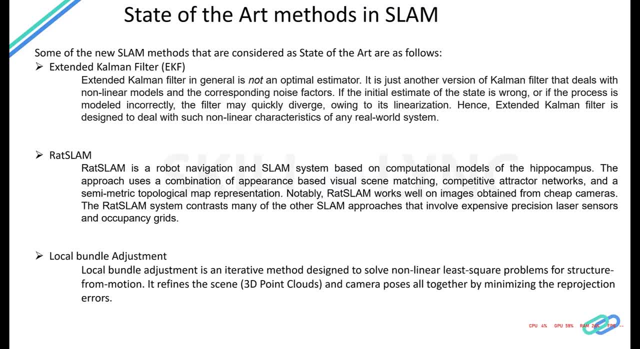 generate the model of the environment. So basically, it basically creates the 3d Point Lodge and defines the scene to that is coming in from the sensor, which is a camera, and then it will try to put yourself on the environment based on this information. um, so i'll keep it, i'll keep this part at a very high level because it's 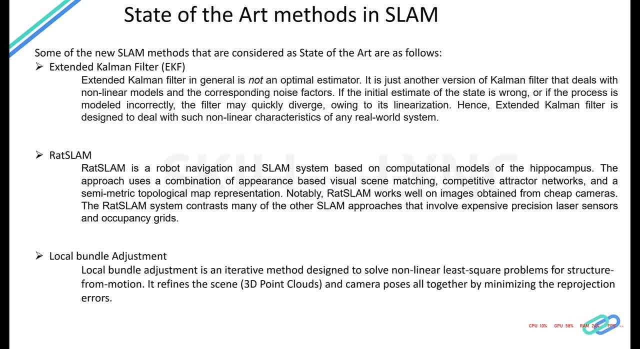 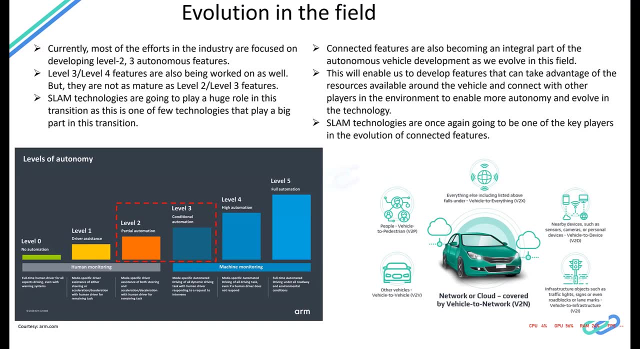 pretty advanced topics and we'll talk about them um once we are starting, once we start with the course. um going to the next one, okay, evolution of slam methods. um, as you know, autonomous vehicles is the booming industry at this time and right now there is a lot of uh. 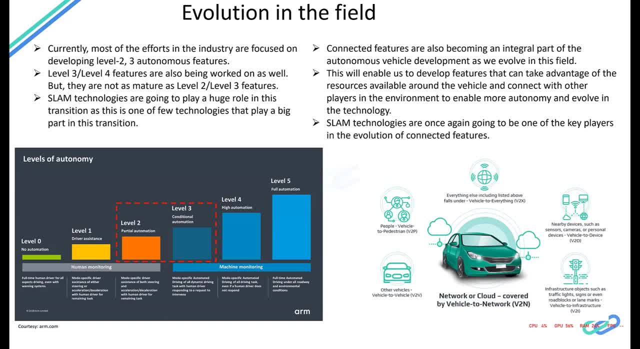 there is a lot of need for autonomous, uh uh, development engineers and, you know, in autonomous space, wherein, um, you have a lot of opportunity in this space. so, um, uh, at this point, where, what, where the industry is that? um, we are mostly focused on job developing, level two and 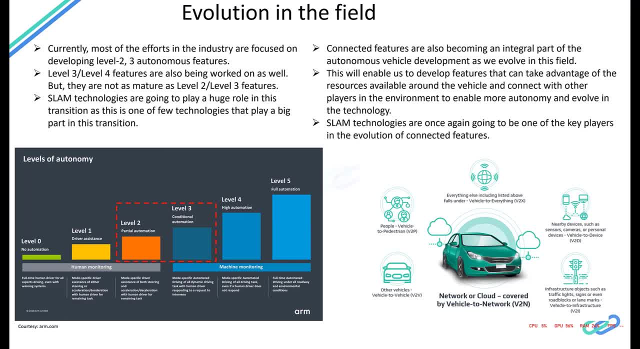 uh level three autonomous systems. i myself work as an autonomous vehicle engineer, so, uh, currently the industry is primarily focused on um level two and development of level two and level three autonomous features. the bottom picture, the bottom left picture, will give you a general um idea of what, what, what are the different levels of automation and where we are with it at. 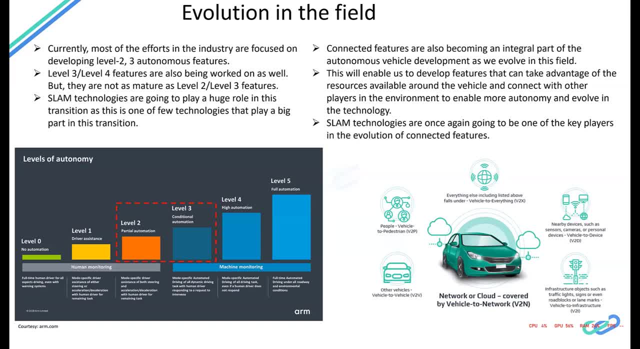 this point. so level two, level three, autonomous features, are basically, you know, partially human. the human is ultimately responsible for it, but the system gives you the ability to automate the driving and all of these different aspects, but not all, not all aspects are automated users. the user is still responsible for, you know, any outcomes of any anything. 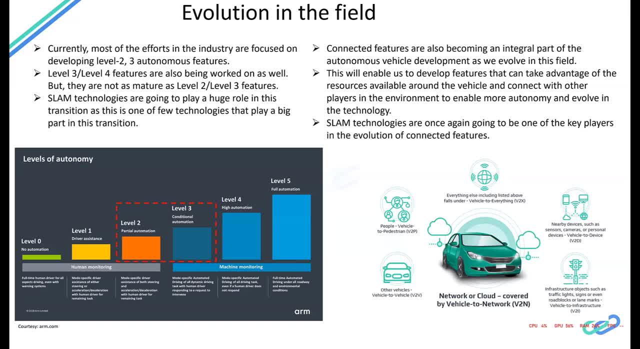 that comes out of using these technologies. so, um, in these different levels of autonomy, as i said, localization and mapping are always one of the major components of any given autonomous systems. because that is the heart of the problem, right? because, um, if you don't know where you are at, if you don't know, 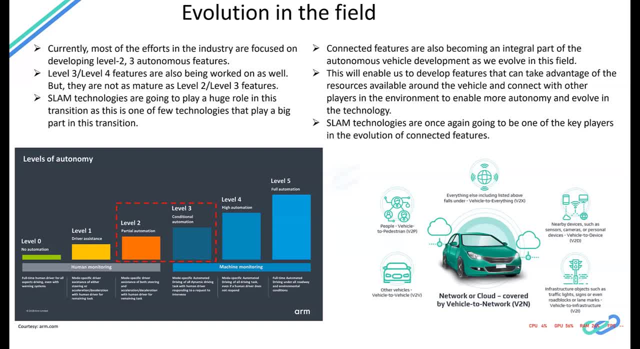 your environment, then there is no autonomous system. um, so slam technologies are always going to be the heart of the problem. so developing strategies to have the news, developing strategies to automatically pursue the system and also use the information to localize in all of these different functions, that has become a challenge. and the slam technologies or the, you know the slam- 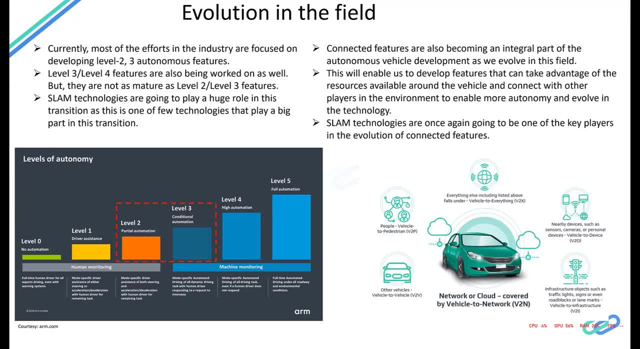 methods are improving on a very high, high pace, and they're playing a very big role in terms of enabling us to get these new technologies okay, um, so the other thing that i will just talk about very quickly is about the connected features. um, connected features are nothing but. 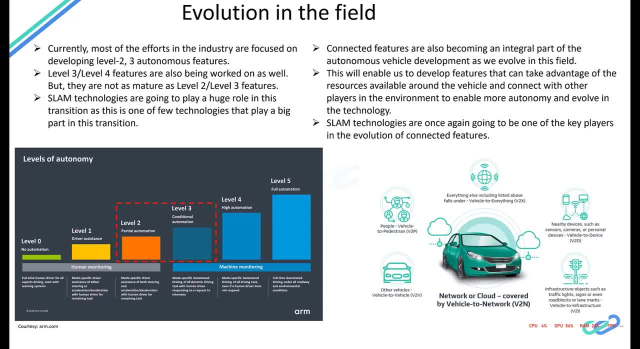 a very simple interface like your phone, as your phone is connected to the network. similarly, your car is connected to the network and then you have a network to vehicle communication and vehicle to vehicle communication. you can you can have an n number of different combinations to it and you use uh information from all these different devices and you know. 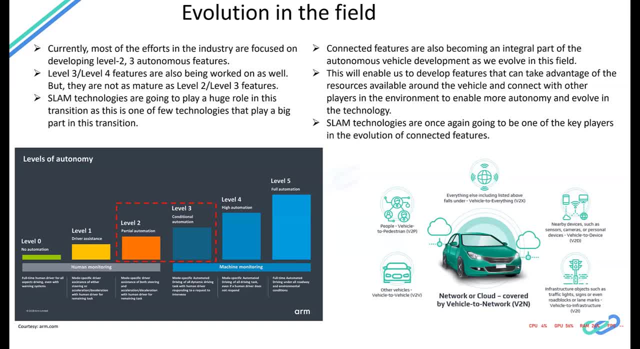 it will help you put yourself on the map, and that's a very uh, a high level introduction to the connected pages as well. and you can also use a multi-ingerector or a multi-area immigration system, which is called the traffic map, and that's uh. that's one of the five applications that are in the 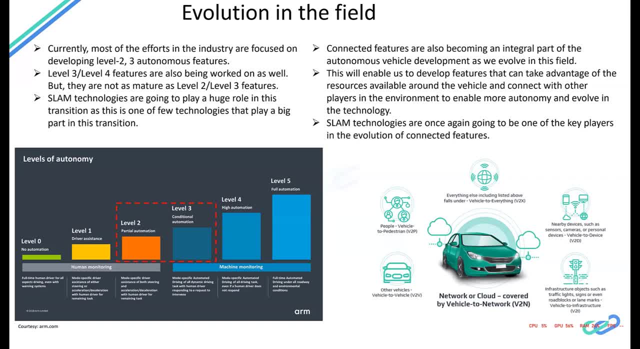 system that can be used for data collection, and then the data has a lot of information so you can actually use it to uh, you know, look at a car, or you can use this as a way of getting information to your route. so you know, that's one of the major um areas where, uh you. 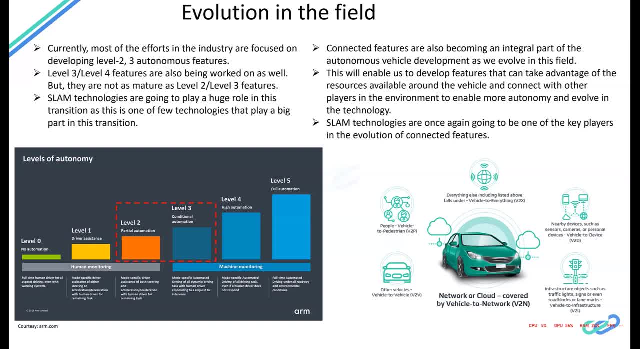 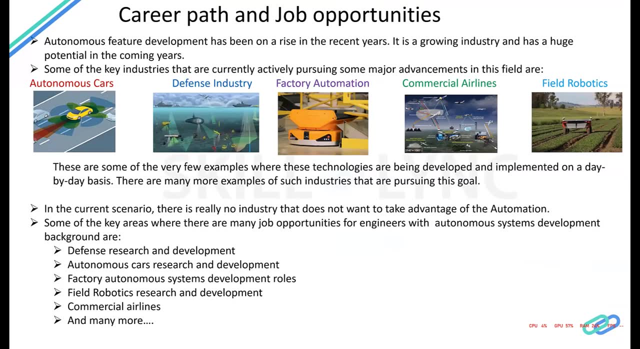 know slam comes in, wherein slam will read the environment- you have 100 cars going on the road, function and put itself locally distance better on the map. so things like this, so this connected features, are also helping us improve upon these different technologies that we are having right now. okay, let's talk about very briefly 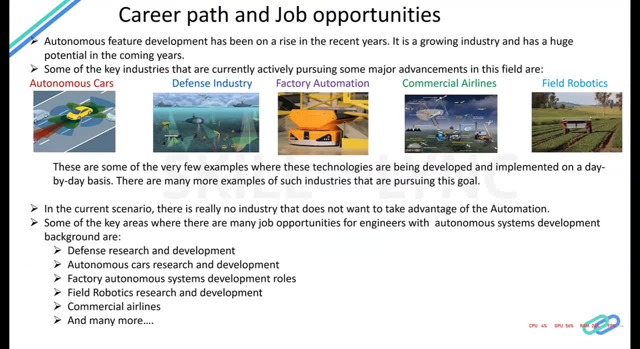 about the career path that you have. think of anything, any system, whether it's cars, whether it's farming, whether it's airplane, or whether it's underwater of vehicles, or whether it's a factored, of our factory environment or home environment. you can take any example and you will always find one. 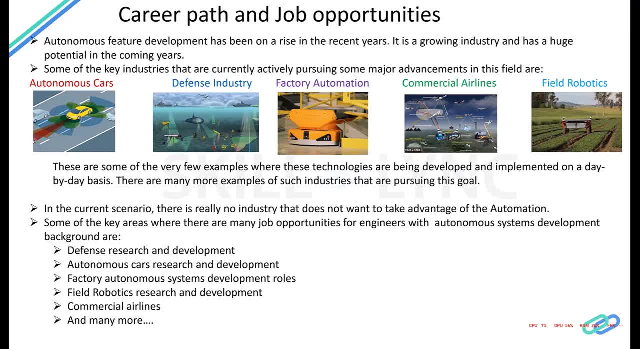 example, for a robotic system. so the opportunities for of being in this space are endless. I mean, I just don't have enough space here to think about it. I'll give you all the examples of you know all these different feeds that you can be in for any for the robot, for being a- well, being a robotic engineer. so 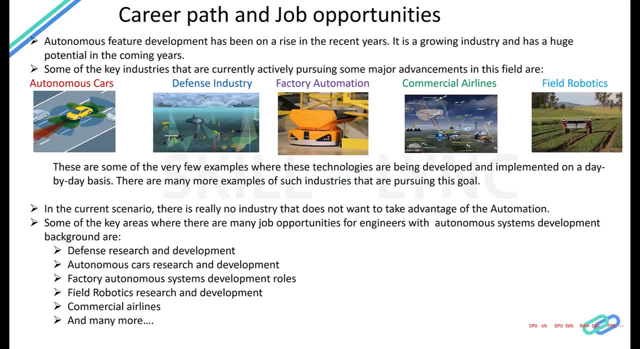 I've given a few examples. autonomous cars is, as I said. it's a booming industry at this time and a lot of countries are passing regulations to move to driver engine less cars like electric cars. and all that and along with electric cars, autonomous vehicles, autonomous features are also.